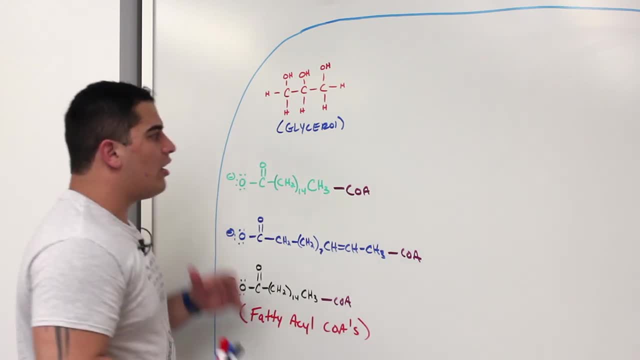 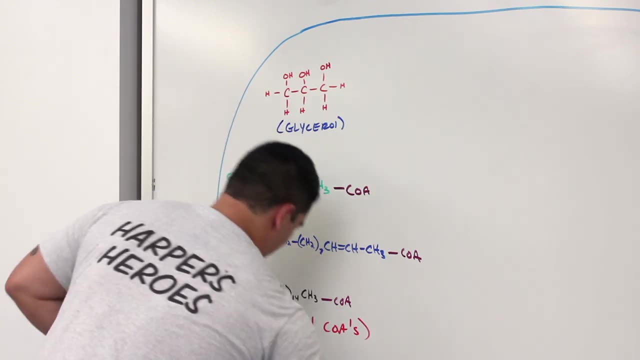 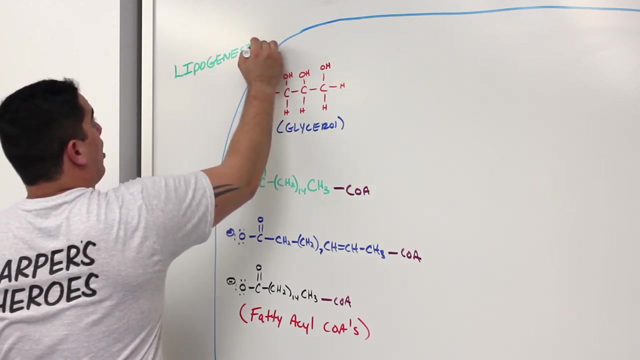 are the constituents to synthesize triglycerides, And you know another word we give for synthesizing triglycerides: they also call it lipogenesis, So another name for it is actually specifically called lipogenesis, And that's what we're going to be talking about in this video. Okay, 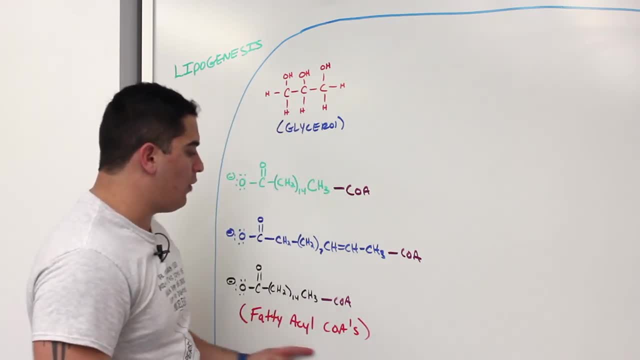 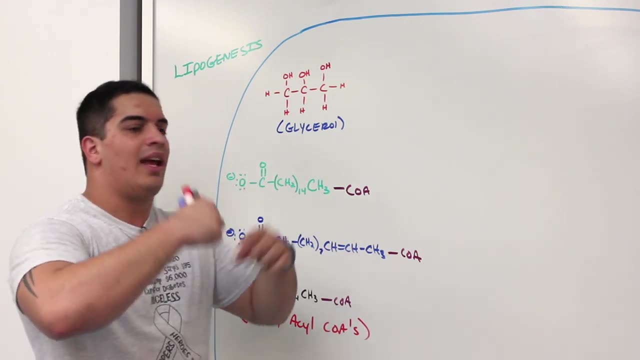 so, if you guys remember, we synthesized the fatty acetyl-CoAs with the malonyl-CoA acting as the precursor, with those fatty acid synthetase enzymes and going through all those different steps with the acyl-caryoprotein and the cysteine thiol. And now that we've done that, we've synthesized- 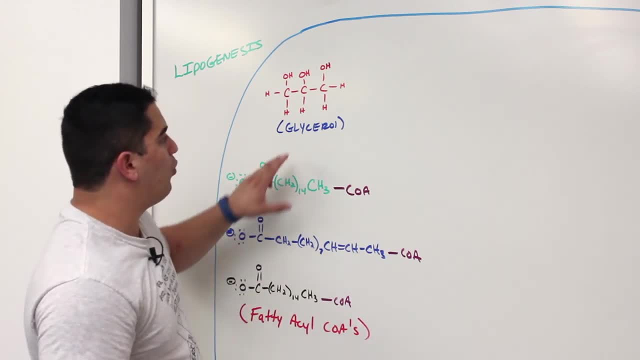 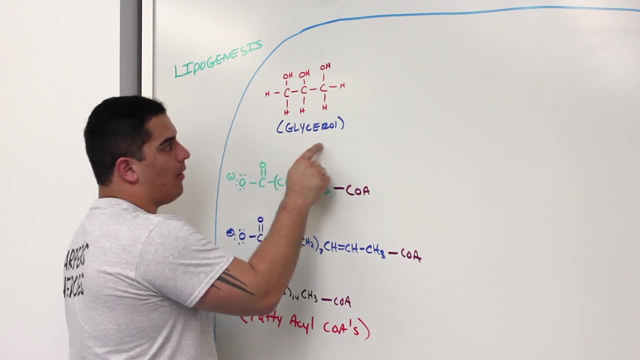 our fatty acids. Okay, now that we've synthesized them, we're going to want to link these guys up. In order for us to do that, though, we need to understand something. We didn't really talk much about the glycerol. Where can that glycerol come from? Well, you know, it can come from just the. 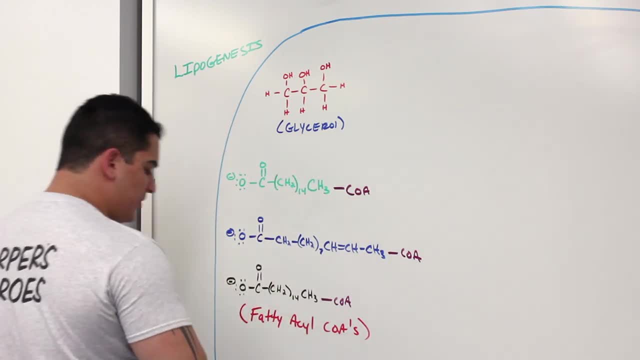 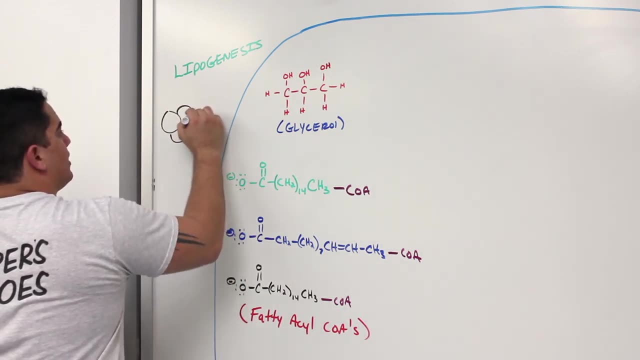 adipose tissue. So if you guys remember specifically from just the adipose tissue, let's say I put over here a couple different adipocytes. So here's a couple of adipocytes And if you guys remember, we could actually break these triglycerides down right And one of the 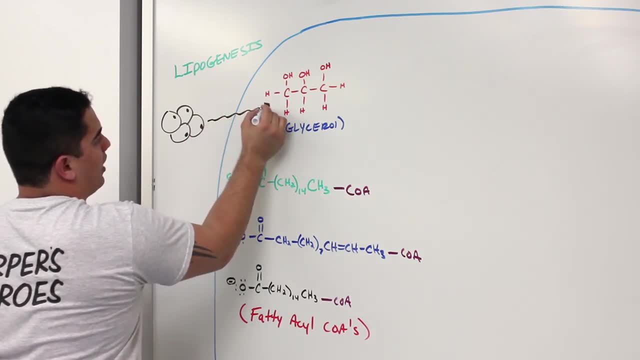 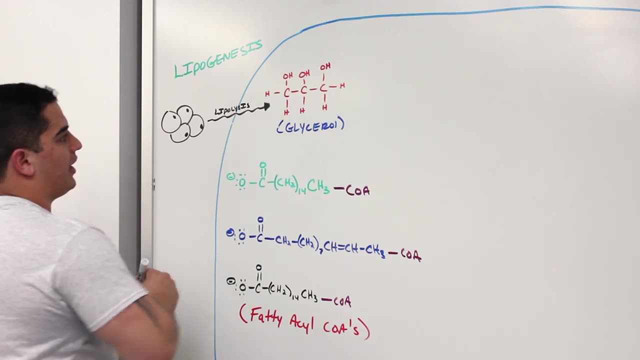 constituents that we can get out of that is glycerol. That's one of the constituents We can get glycerol, And what was this from? This was from lipolysis. Where else can we get the glycerol? You know, from the glycolysis. 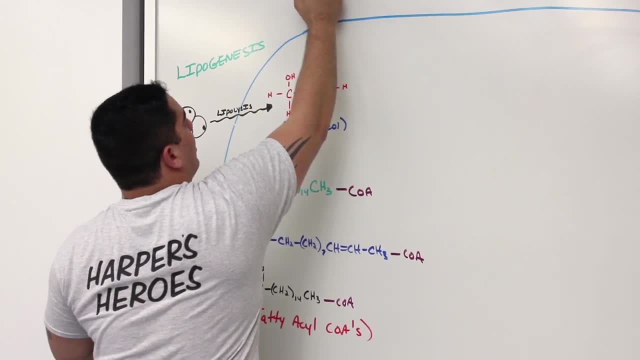 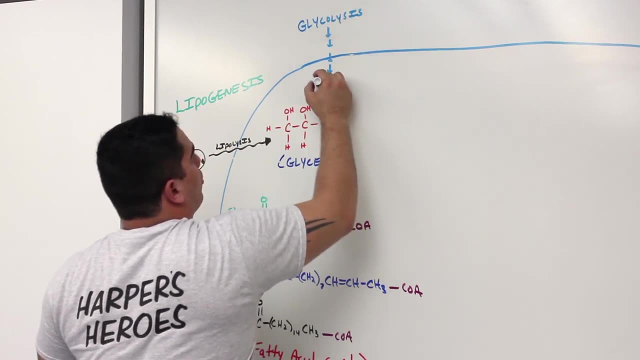 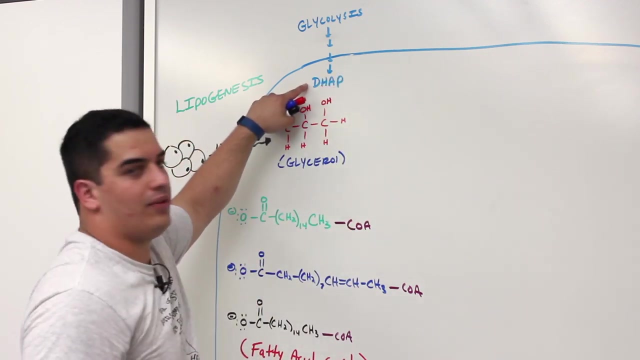 there's a specific point in the glycolysis pathway. So let's say, here I have glycolysis pathway And a specific point in the glycolysis pathway is you form a molecule called dihydroxyacetone phosphate And that dihydroxyacetone phosphate, if you guys remember, he was able to be converted. 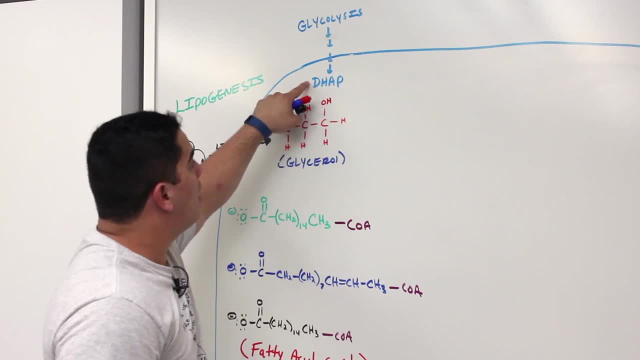 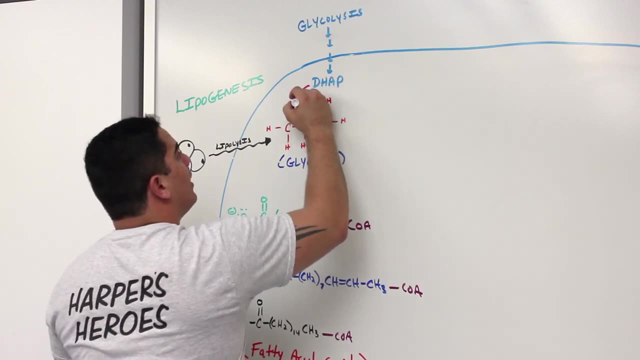 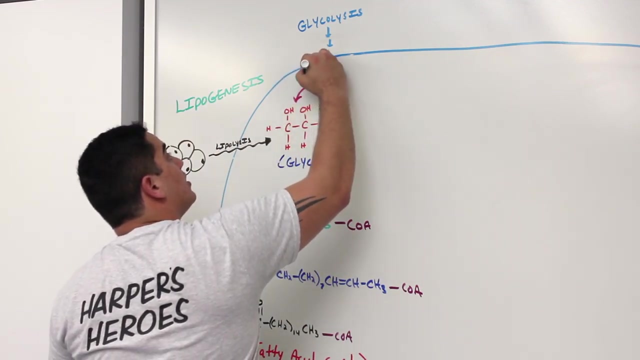 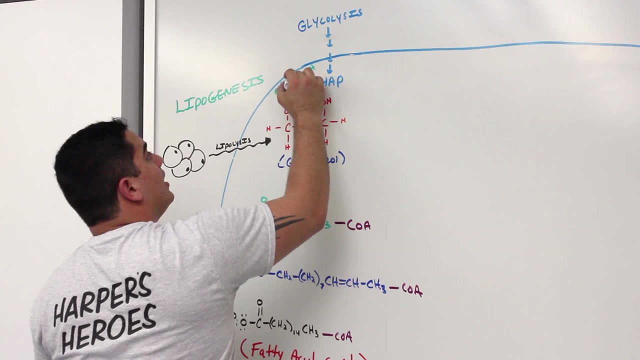 into this glycerol molecule, So let's show how this happens. So this dihydroxyacetone phosphate can be converted into glycerol. In order for that to happen, though, I need to take and drop off some hydrides, So I need to take NADHs that I've generated and convert them into NAD-positive, So 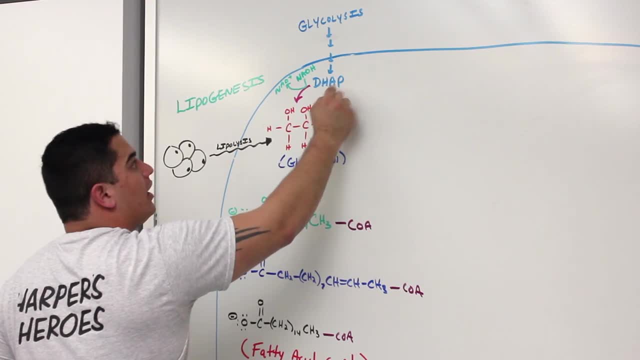 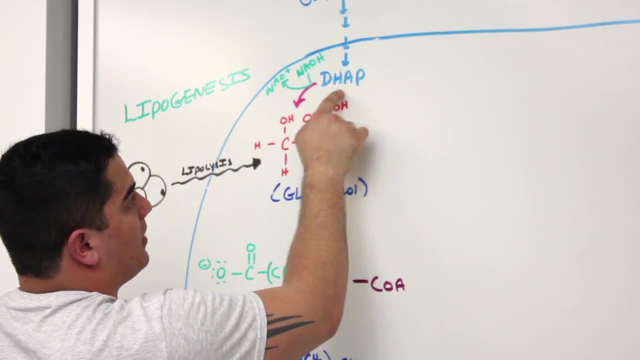 what am I doing? I'm dropping off hydrides onto this dihydroxyacetone phosphate and converting carbonyls into alcohols. But another thing is this guy has a phosphate on a specific carbon. We're going to have to put a phosphate on one of these phosphates Now that son Kickstarter to 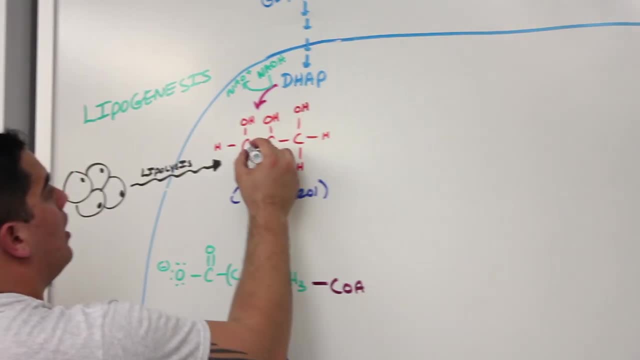 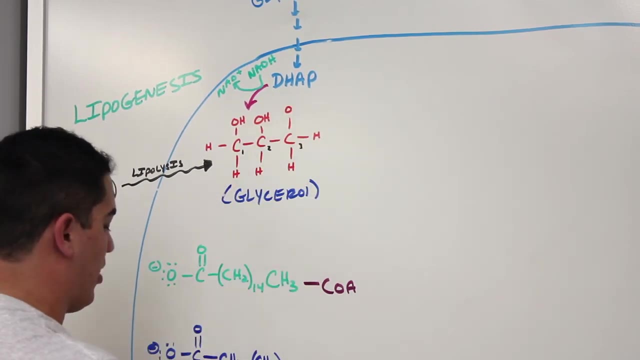 of this guy's carbons too. so if we were to number this glycerol one, two, three carbon chain right on the third carbon of the alcohol, there should be a phosphate group coming off of it. so what should be coming off here? there should be a phosphate group coming off. 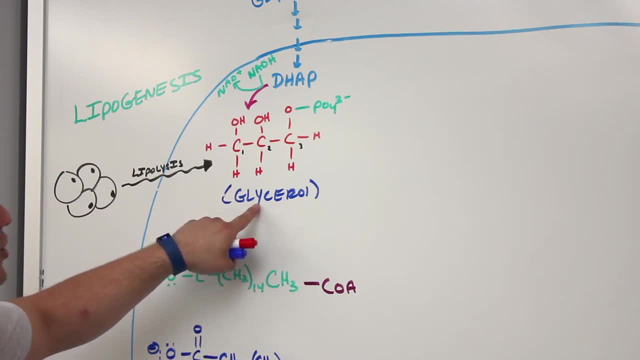 so now, what do we specifically call this? we call this glycerol three phosphate. that's what we really should call it, right, we should technically call this glycerol three phosphate. before we do that, though, let's actually show that in an actual single step reaction. let's do that in a single 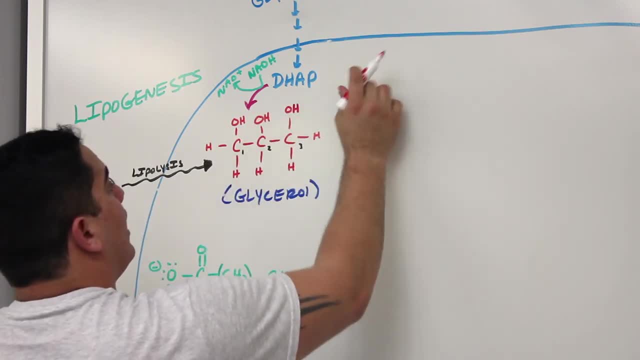 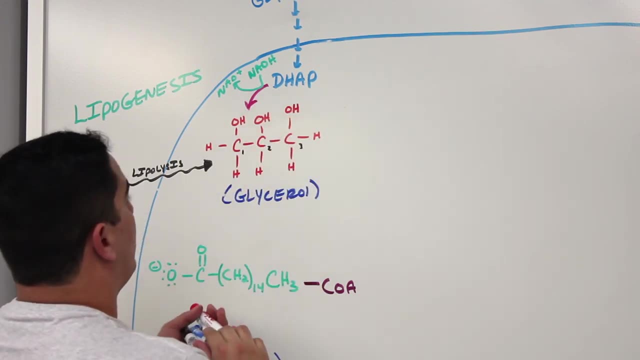 step reaction. so let's put the alcohol back on here and then let's use a specific enzyme. technically there's technically a specific enzyme that can do this step right here. we're going to show it as a separate step here. i'm going to take this glycerol and i'm going to have a special. 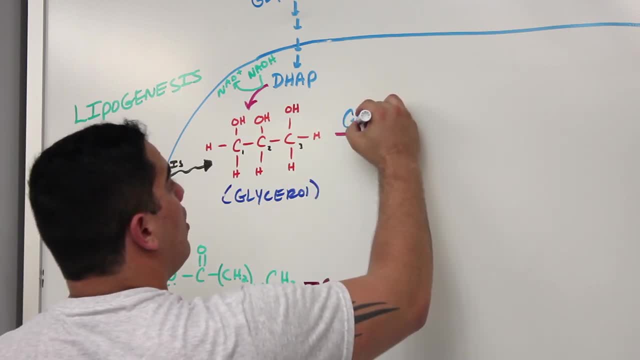 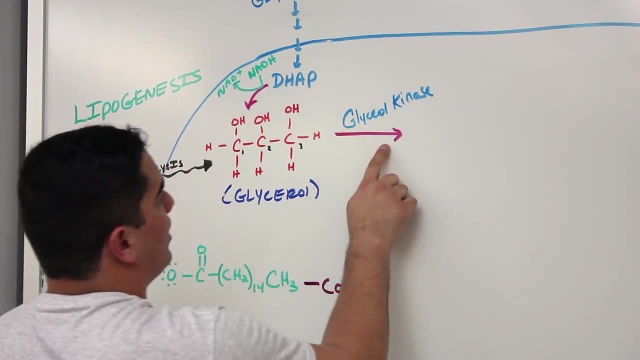 enzyme, and this enzyme is called glycerol kinase. it's only present in the liver right, and what this glycerol kinase is going to do is it's going to put a phosphate on the third carbon of glycerol. so let's say, i take this phosphate here and i feed it into this reaction here. okay, 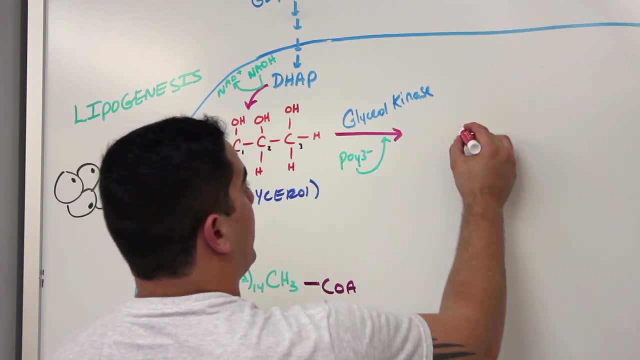 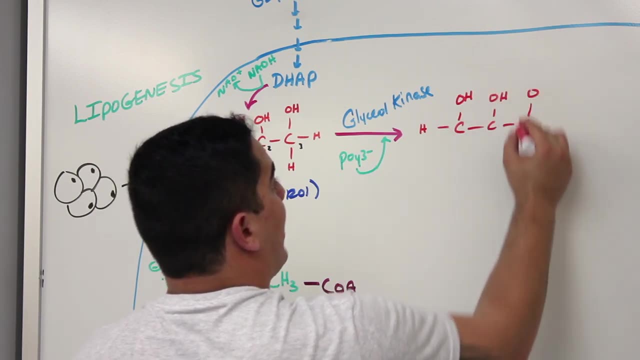 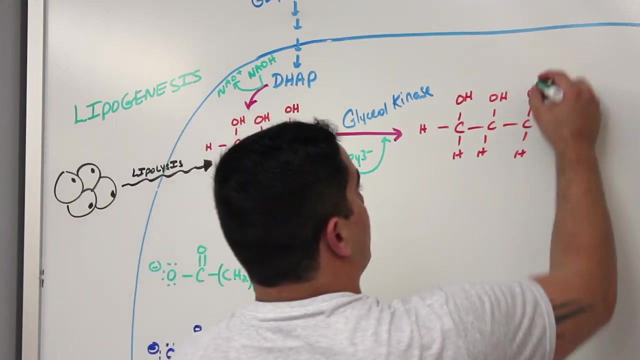 now, what is going to happen? now, let's draw our glycerol over again here, our three carbon unit here, right with our hydrogen there, our oh here, carbon, oh carbon. but then we have the oxygen. there. let's draw all our hydrogens. and then now, what should be linked to this oxygen? guys, there should. 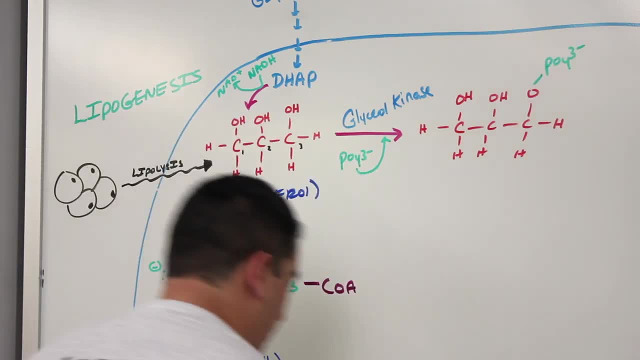 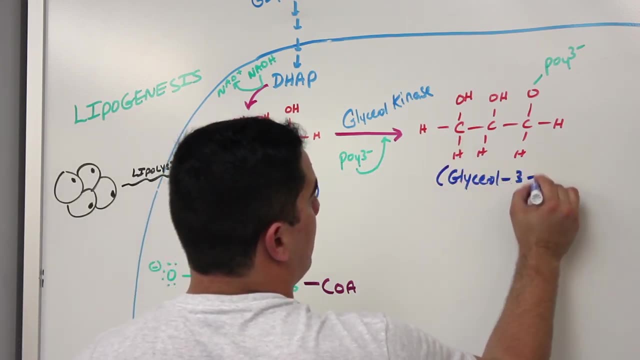 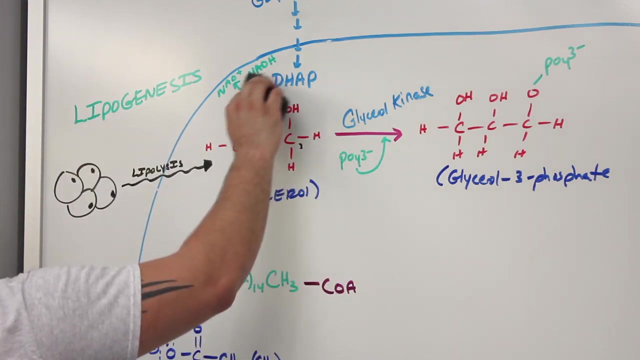 be a phosphate. now what is this molecule here called? this molecule is called glycerol 3-phosphate. so technically, if we really want it to be particular, we could actually erase this step here from dhap going to glycerol, because technically, if you guys, 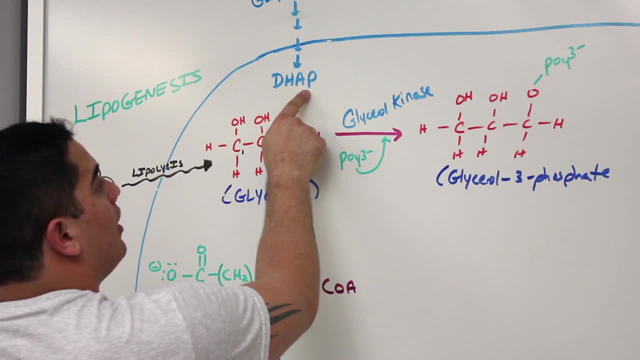 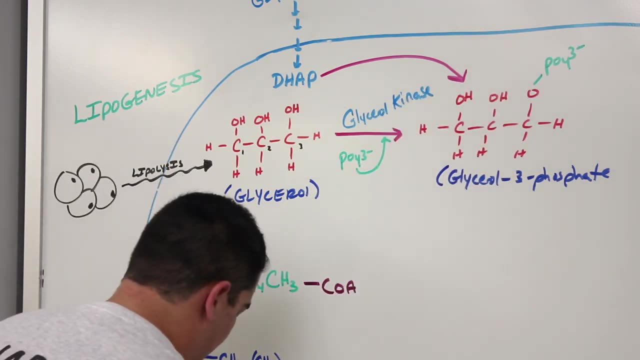 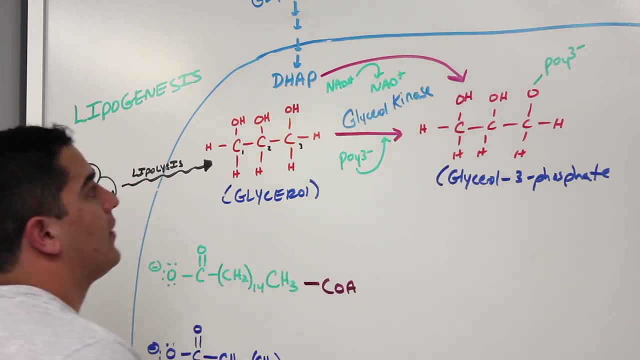 know, dhap is actually converting into glycerol 3-phosphate, and it's actually pretty simple. what you're gonna be able to do is, in a physical way, we're going to dramatically increase the glycerol requirement, back up to the glycerol requirement, and then 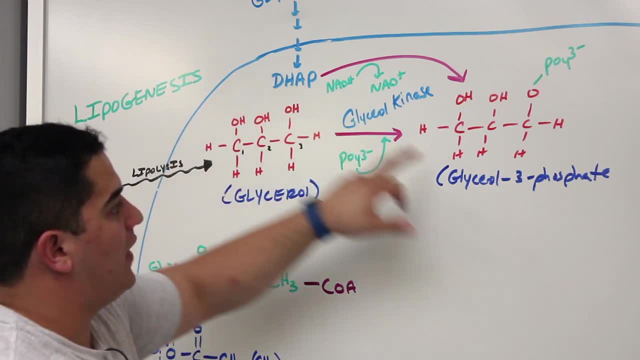 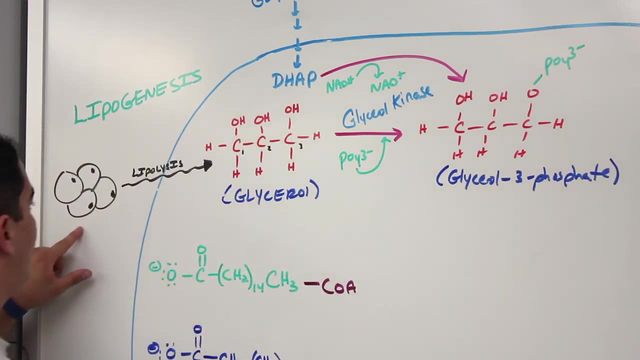 we're going to put in which are actually two different catalysts, and so we're going to draw off the four Member stesso to this glycerol three phosphate, which is the hydrogen dioxide, and then we're going to separate out these two three phosphates, right, right, so we're going to 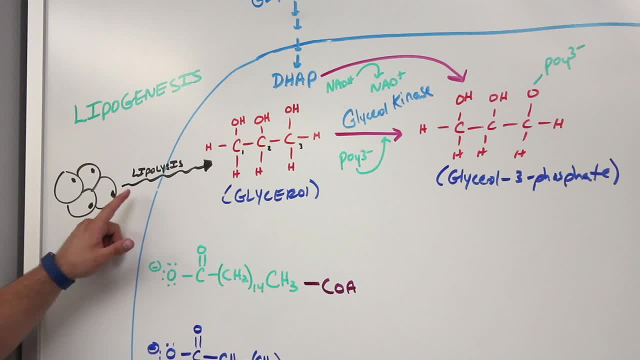 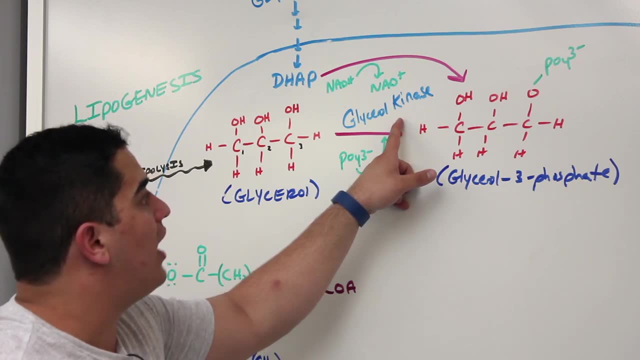 arrange. these two should actually show that over here. and then again, what are we generating in this? What we can do is we can use the glycerol here, and I have an enzyme called glycerol kinase, And glycerol kinase can convert glycerol into glycerol 3-phosphate. 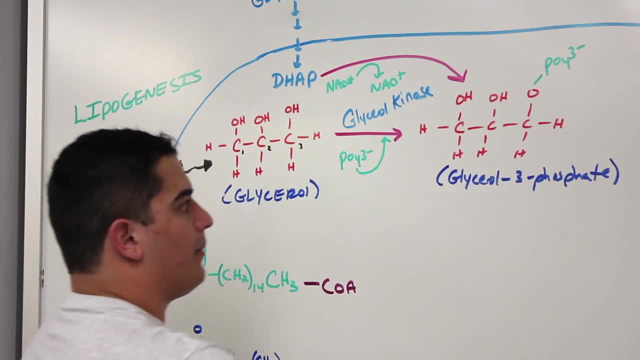 Okay, now the next thing that we have to do here. Then we have to take this glycerol 3-phosphate and combine it with each one of these fatty acetyl-CoAs. So now what I'm going to do is I'm going to draw the glycerol in a large view here. 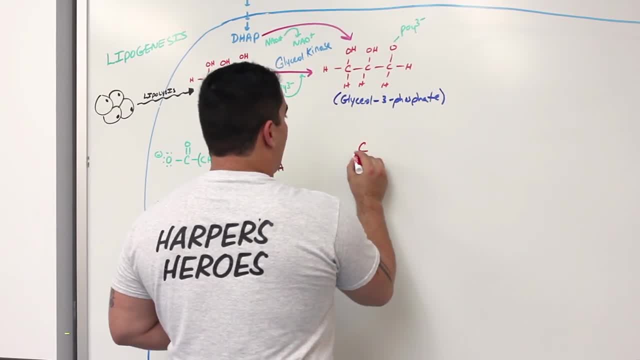 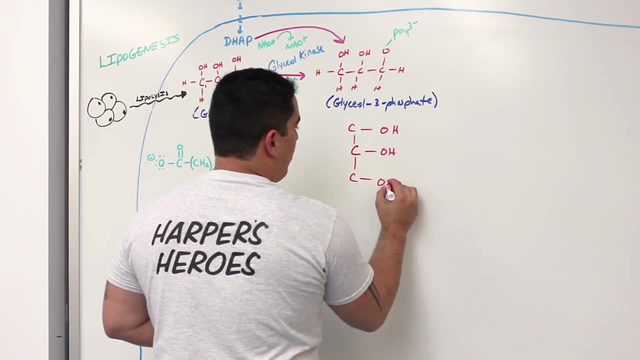 So now we're going to take this glycerol step by step here. So let's say that here we have our carbon. I'm going to draw it like this now And I'm going to put my OHs right here And again. on the third carbon, I shouldn't have an OH. 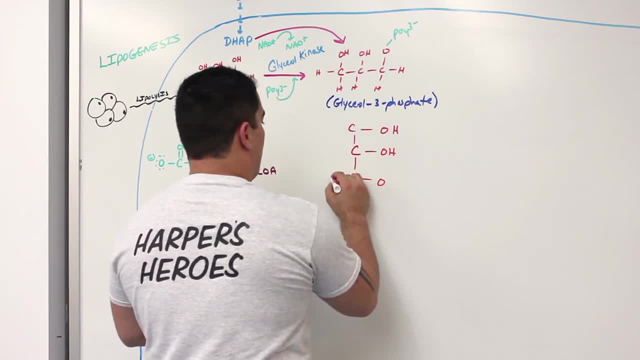 I should have a phosphate group coming off. Let's draw all the hydrogens coming off of this puppy. Okay, there's our hydrogen there. There's our hydrogen there. Okay, and again, let's number it, just so we know exactly where we are. 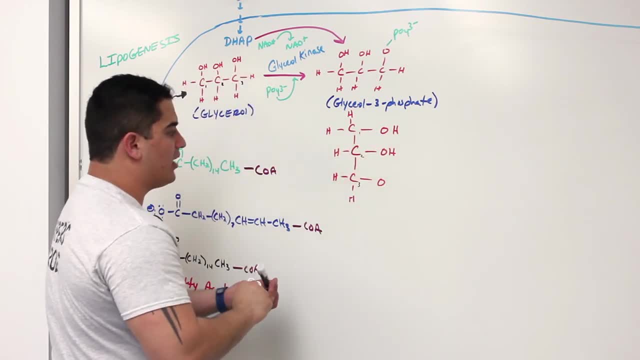 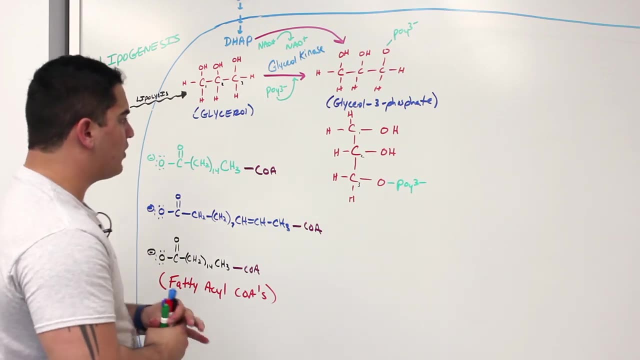 One carbon, two carbon, three carbon. But you would know that because on the third carbon there is a phosphate group. Okay, Now, Now, what's the first step? The first step is: I'm going to number each one of these fatty acids. 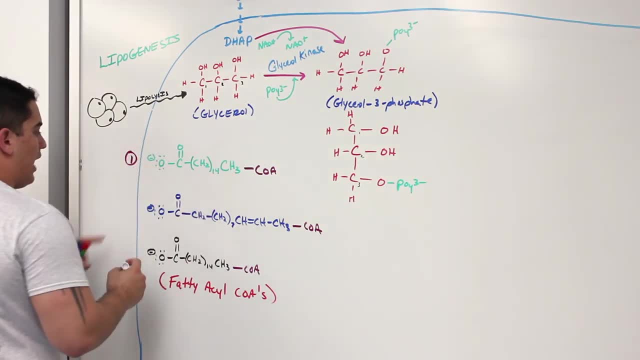 I'm going to number this fatty acetyl-CoA number one, I'm going to number this fatty acetyl-CoA number two And this fatty acetyl-CoA number three, Because we're going to add each one of these on in sequence. 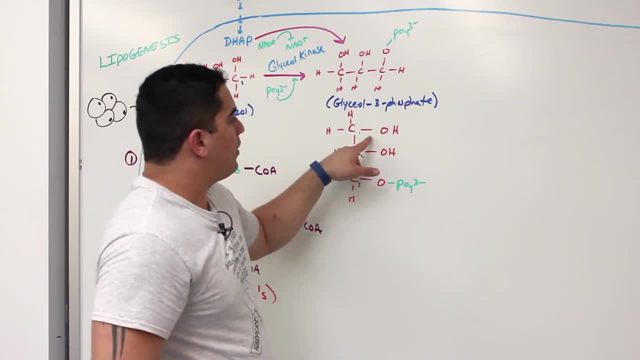 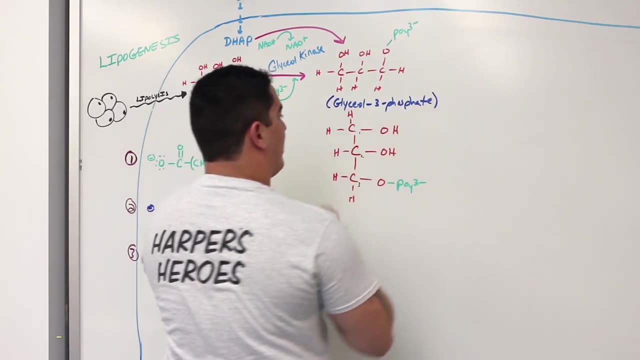 Because it's very particular in the way we have to do this. So the first thing we're going to do is we're going to add this fatty acetyl-CoA onto the number one carbon. So now I'm going to take this guy here and I'm going to add it onto that one carbon. 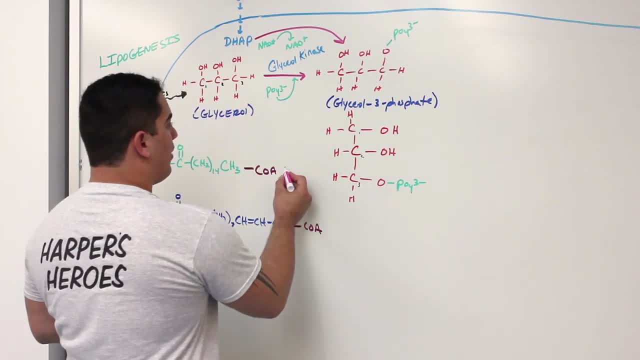 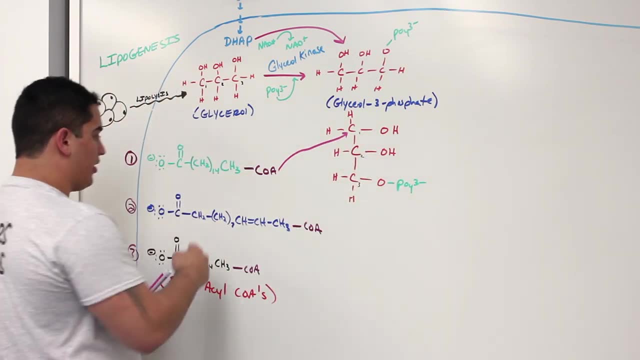 So let's show that. So this guy right here is going to come in and it's going to be added onto that one carbon. Okay, Then, if you want to be particular, this guy here would be added onto the second carbon, And this guy right here would be added onto the third carbon. 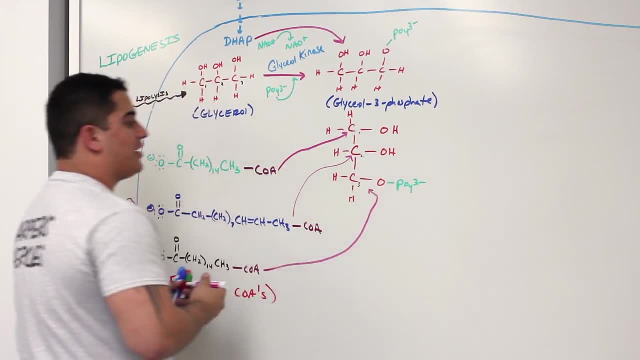 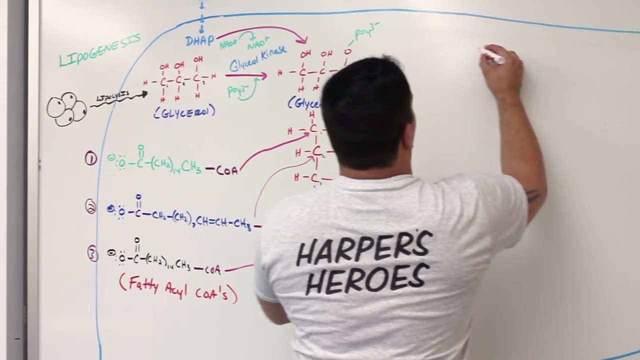 But there would have to be a specific sequence of actions of how this is happening. So now, what we're going to do is we're going to show this in a sequence of steps of how it's going. Okay, So now let's have our carbon group here. 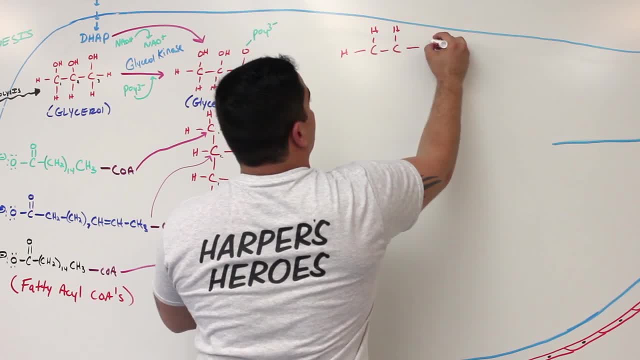 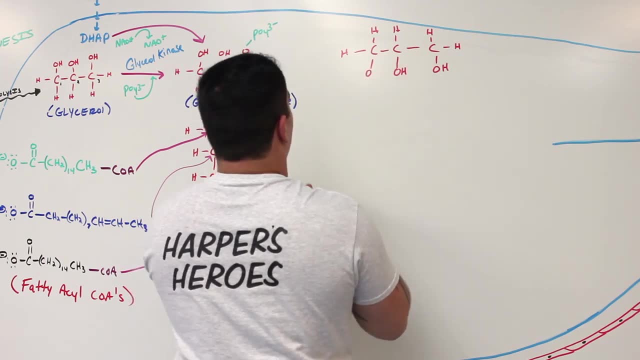 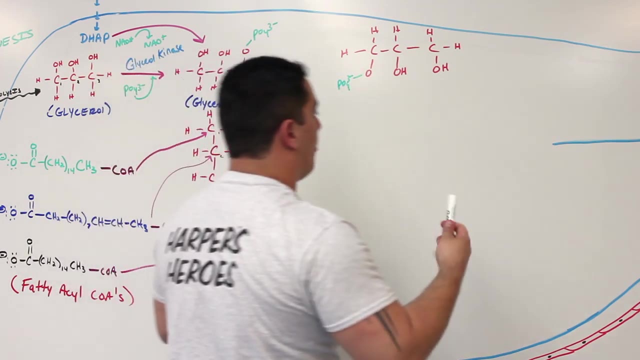 Hydrogen, hydrogen, hydrogen, hydrogen, hydrogen again, And then let's have our OH here, OH, and then again our oxygen with the phosphate group. Okay, So let's take that first fatty acetyl-CoA that we're going to call fatty acetyl-CoA number one. 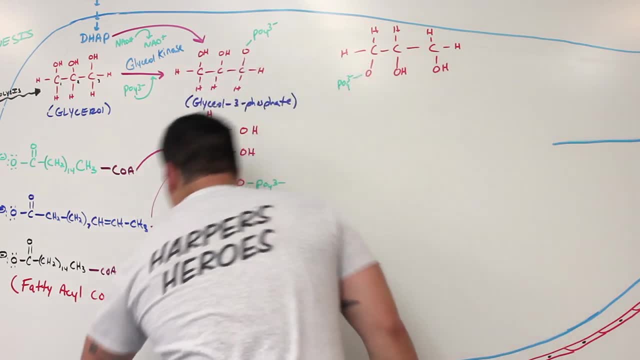 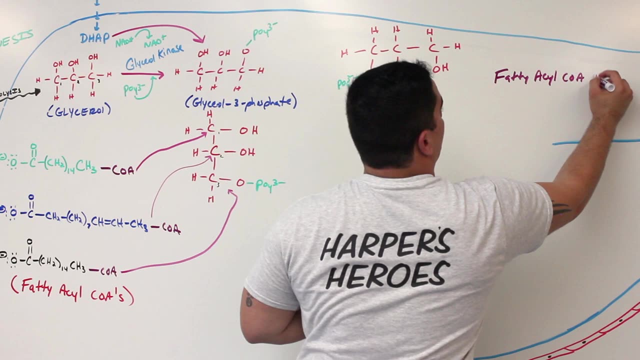 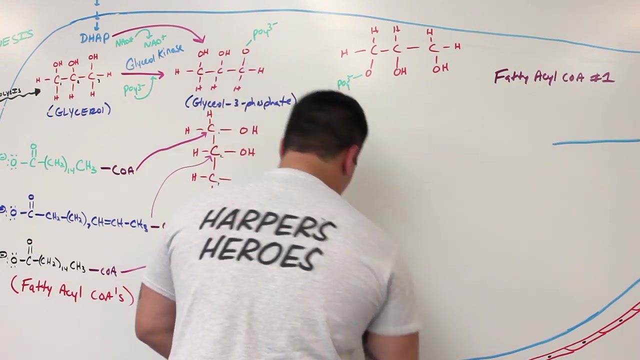 So we're not going to show that whole structure, We're just going to say specifically, this one is going to be fatty acetyl-CoA number one. I'm going to add this guy into this guy here. So I'm going to take and fuse these two guys together. 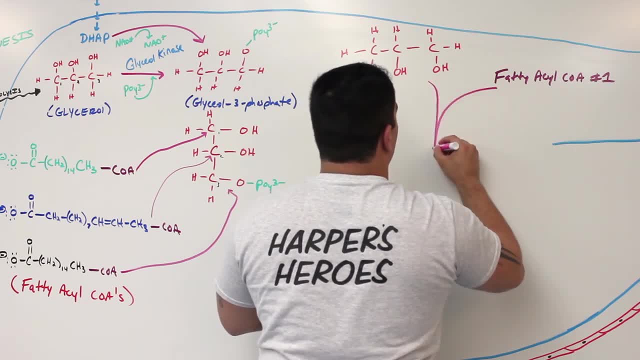 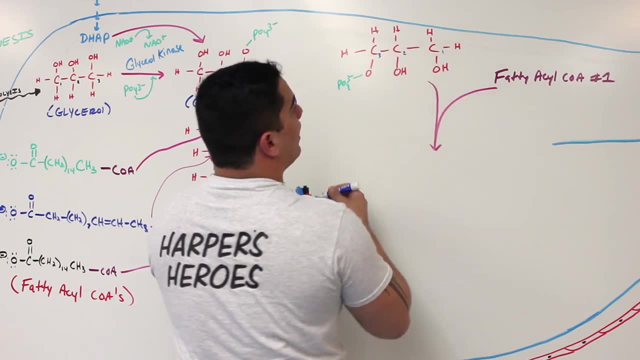 But when this guy reacts, with this guy we're going to specifically again. let's get our carbon straight here again. This is carbon one, carbon two and carbon three. This fatty acetyl-CoA number one and this glycerol is going to be acted on by a special enzyme. 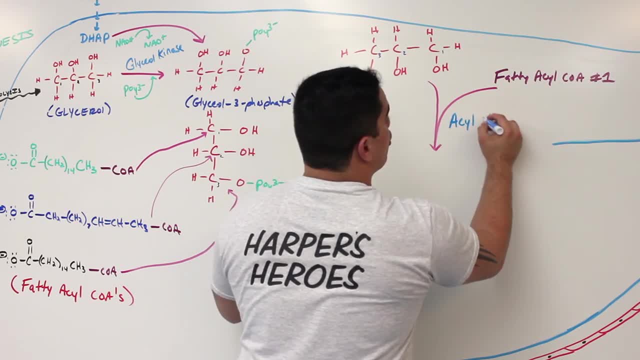 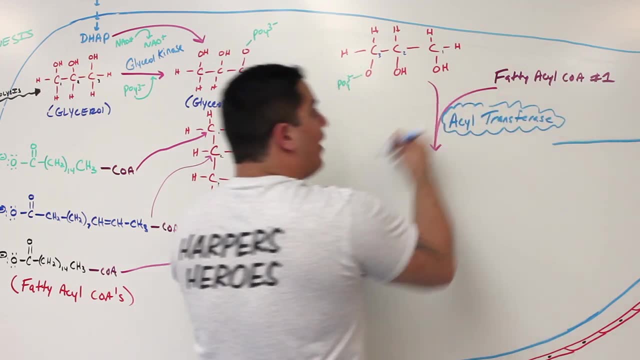 And this enzyme is called acyltransferase. Okay, So it's not hard to remember, because this enzyme is transferring a fatty acetyl-CoA on here. And what are you going to lose? You're going to lose a coenzyme A out of this reaction. 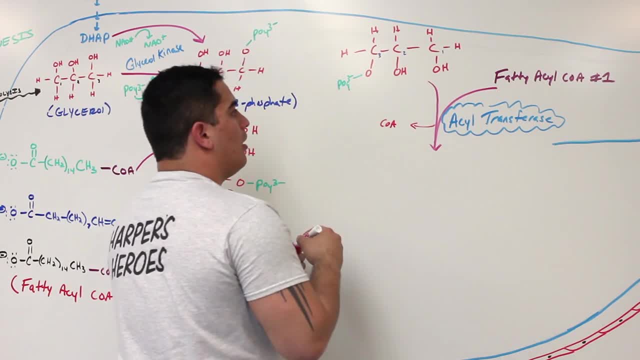 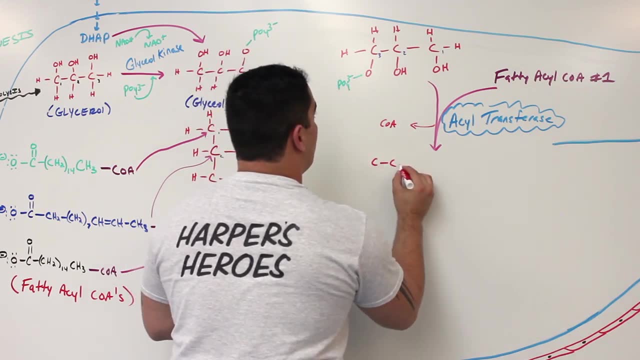 So you'll lose a CoA, But this fatty acetyl-CoA number one is going to be added onto the number one, carbon. So now let's show that. So boom, boom, And again I'm going to have my hydrogen here, hydrogen here. 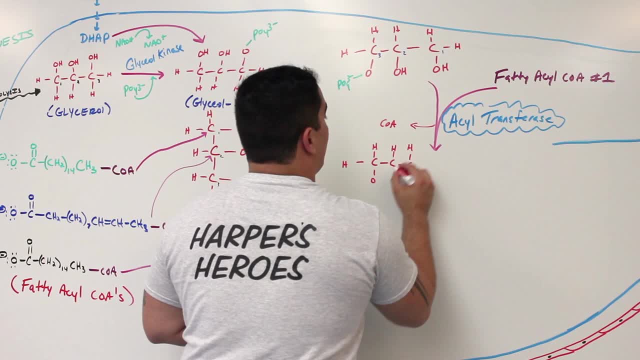 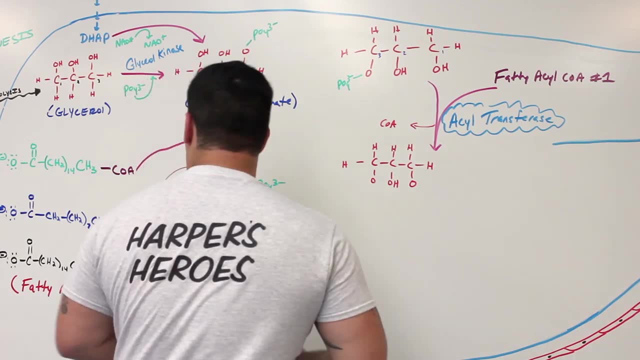 Still going to have my phosphate group there. That hasn't changed. But now, look what's going to be different now On the first carbon. I'm going to have my oxygen there. But now, what am I going to have? I'm going to have this fatty acetyl-CoA added to it, but without the CoA. 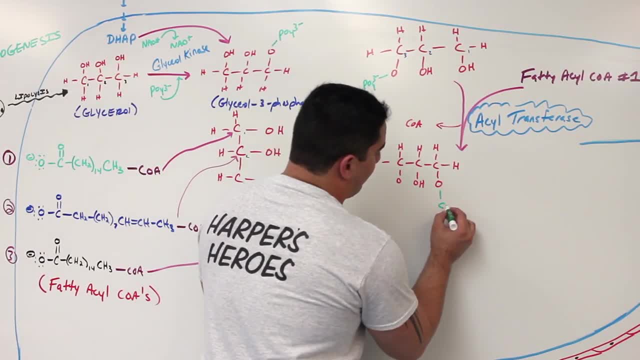 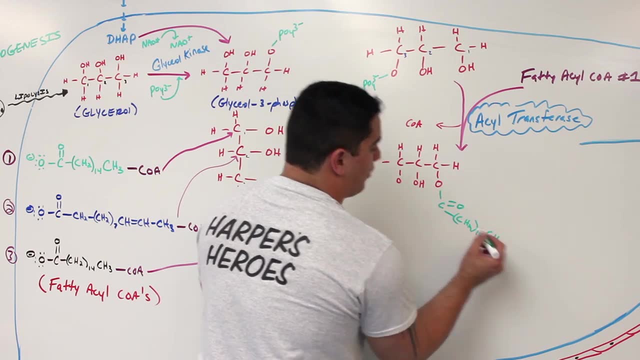 So let's draw that. So now, what am I going to have? I'm going to have carbon double bond oxygen And this is going to have a CH2, 14 carbons like that with a CH3.. What do I call this molecule? 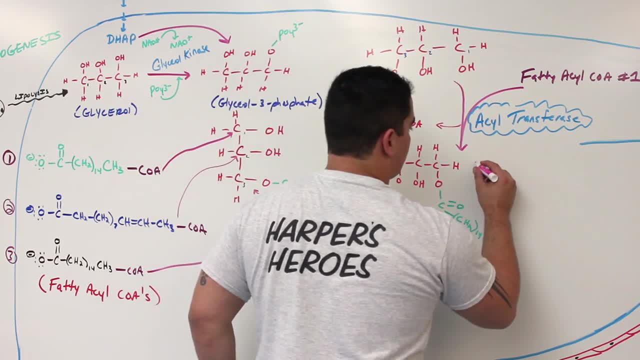 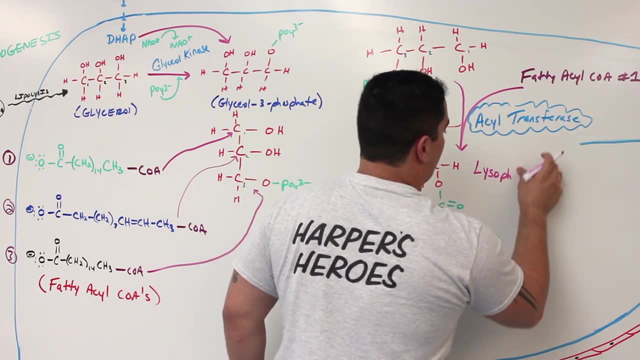 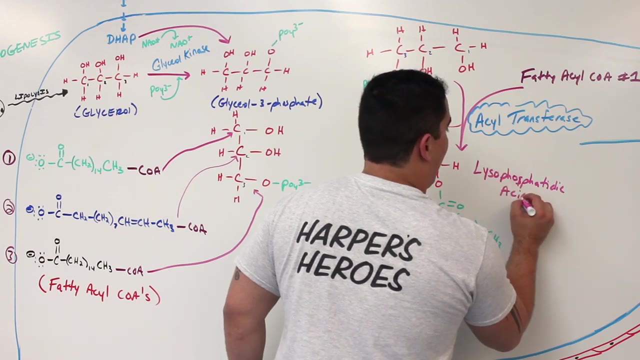 This molecule is called lysol. This molecule is called lysophosphatidic acid. So this first molecule that we just formed is called lysophosphatidic acid. Okay, so that's the first one that we formed. We formed our lysophosphatidic acid. 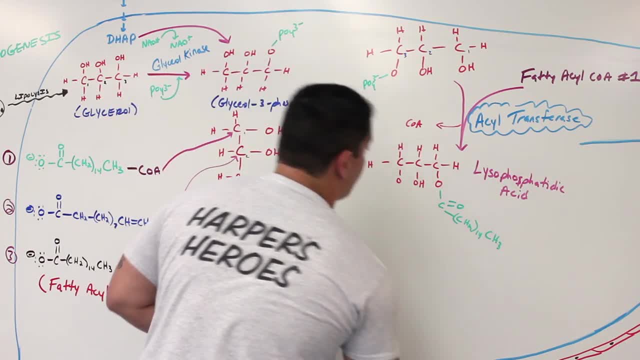 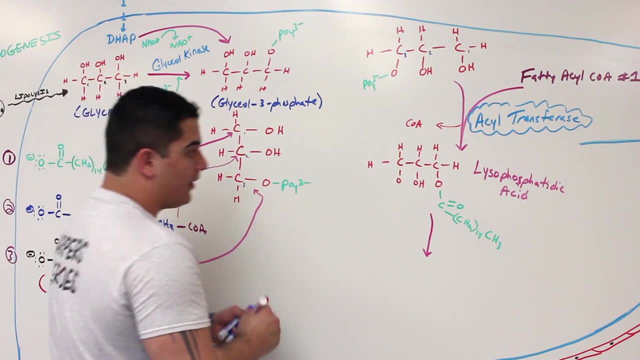 Okay, now that we've formed our lysophosphatidic acid, let's do the second step. So now in the second step, it's just going to be the same thing. So look here, in the second step, In the second step, what am I going to be adding here? 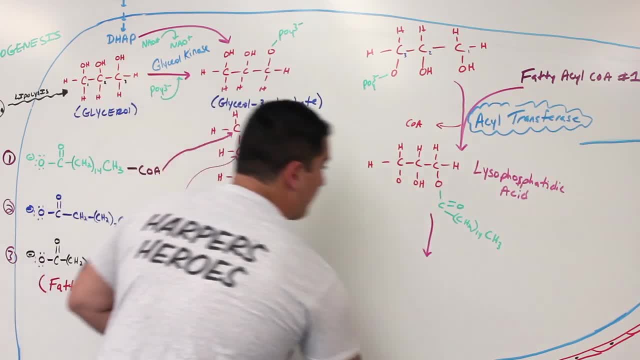 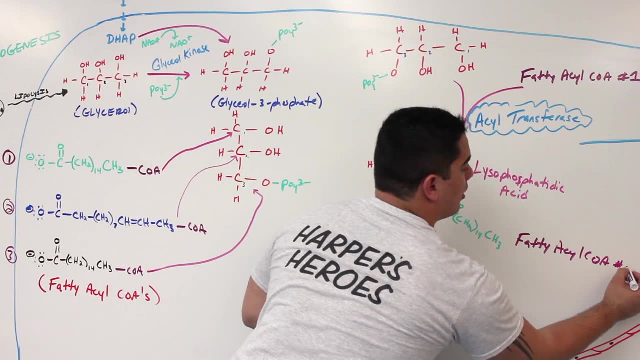 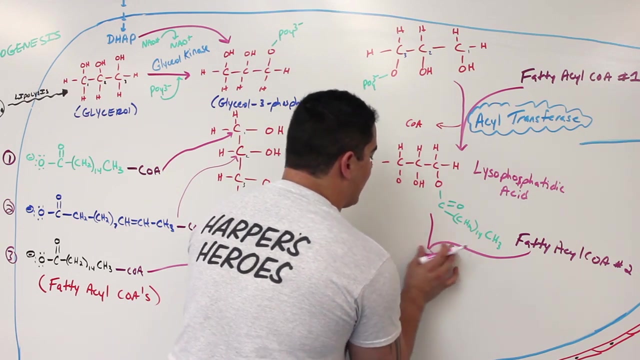 I'm going to be adding the second fatty acetyl-CoA. I'm going to add this guy. So I'm going to add fatty acetyl-CoA number two. So these two guys are going to react, But again, the enzyme that's catalyzing this step here is still going to be an acetyltransferase enzyme. 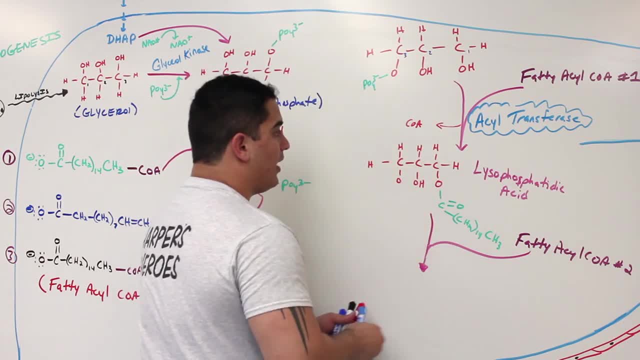 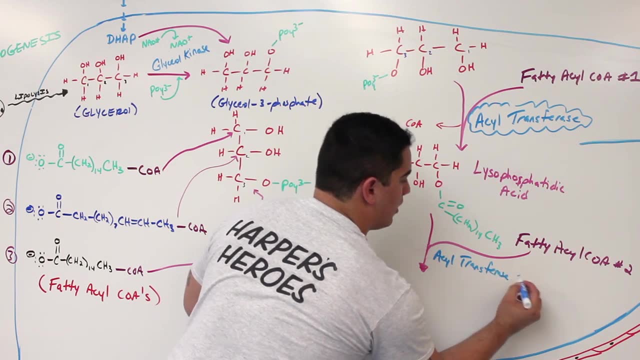 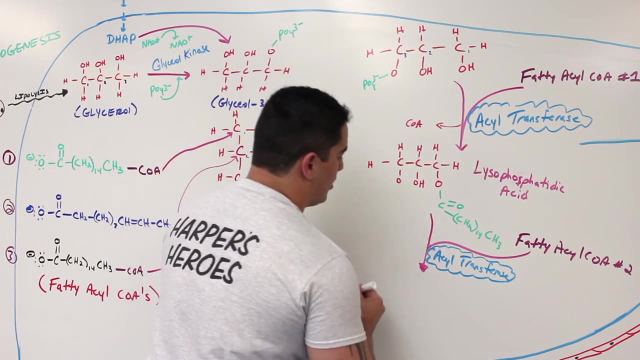 So what is the enzyme triggering this reaction to occur? Again, the enzyme is going to be specifically an acetyltransferase enzyme. Okay, and again, what are you going to lose out of this step? here, You'll lose a coenzyme A. 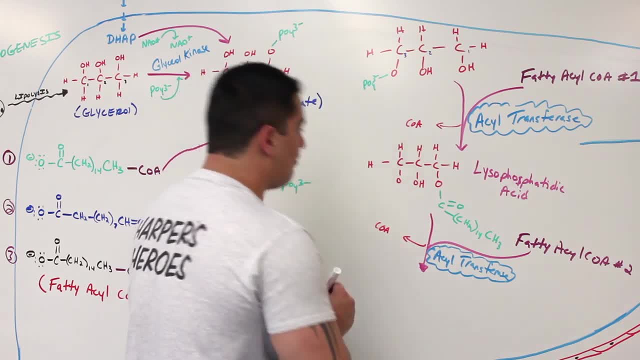 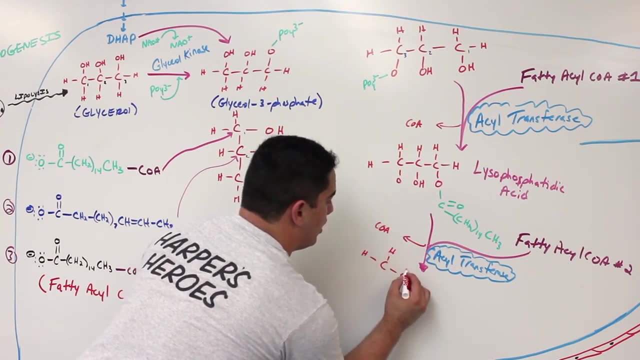 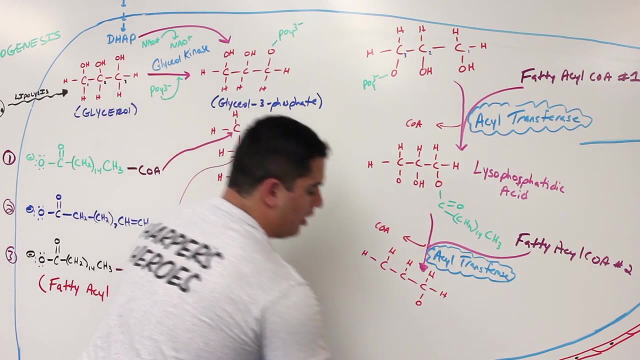 So out of this will come a coenzyme A. Now let's draw this new molecule right here. So now we're going to have our carbons of all the hydrogens attached here again. But now, if I redraw this guy here, we have our first glyphosate, the fatty acid, added on here. 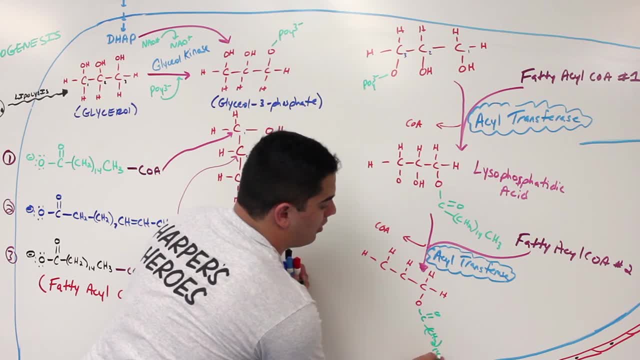 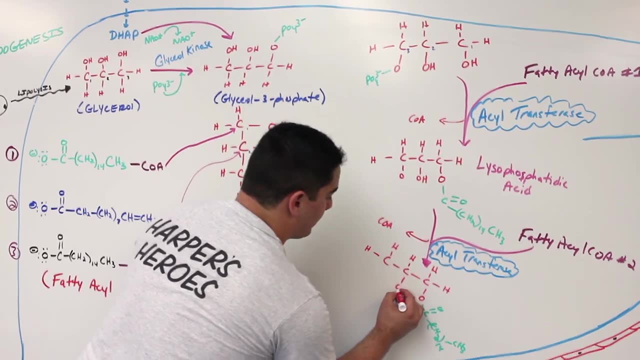 Okay, And then what are we going to have? We're going to have another fatty acid added on. So now let's add this next fatty acid. So how does this reaction occur? I'm going to add in this guy here: 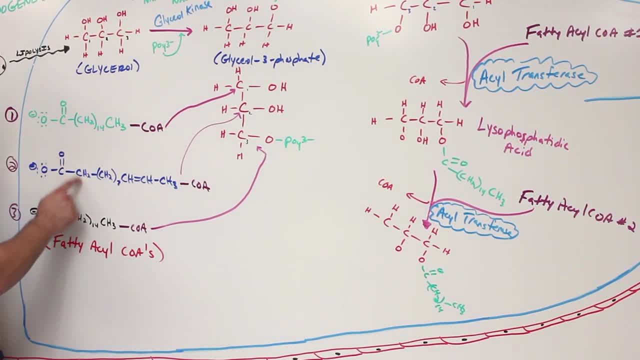 But here's the key thing: What do you notice the difference between this guy and this guy? This guy has double bonds, So he's an unsaturated fatty acid. This is a saturated fatty acid. Saturated just means that it has no double bonds. 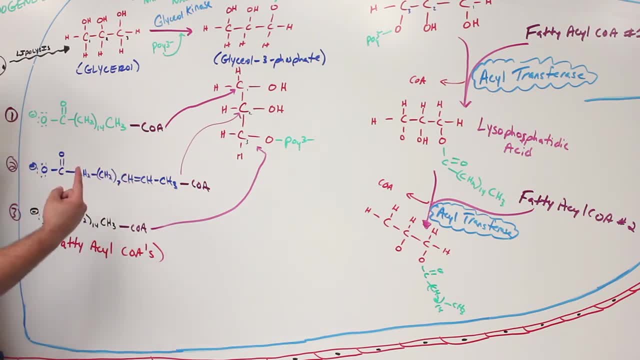 Unsaturated means it has a double bond. If it's monounsaturated, it has one double bond. If it's polyunsaturated, it could have many double bonds. The critical thing is that the second fatty acid added has to be unsaturated. 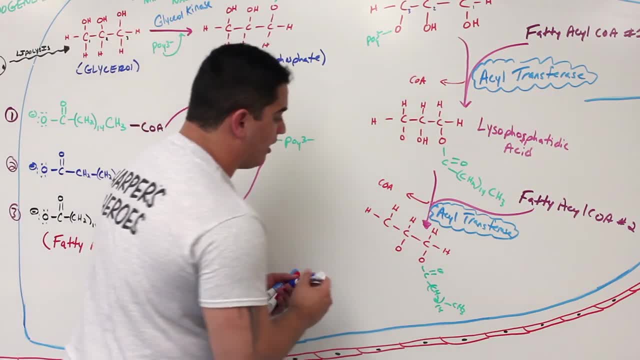 Okay, So now we're going to add on this second fatty acid, but it has to be unsaturated. So now let's add that on. So now we're going to have again the carbonyl, And then what does it have? 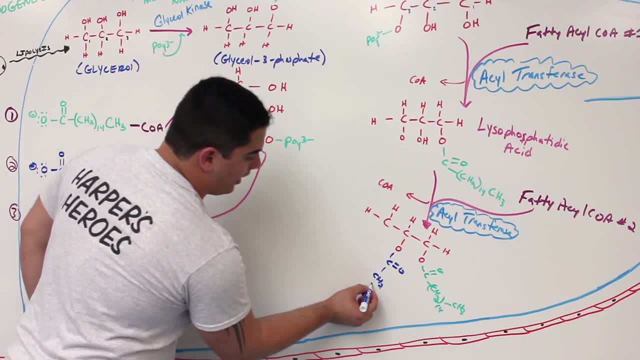 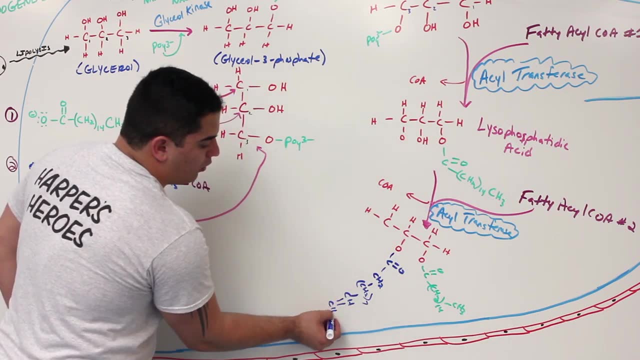 It has a CH2.. Then it's going to have a CH2, but seven of them like that. Then you're going to have a carbon which has a double bond with another guy, And then what? Then you're going to have a CH3.. 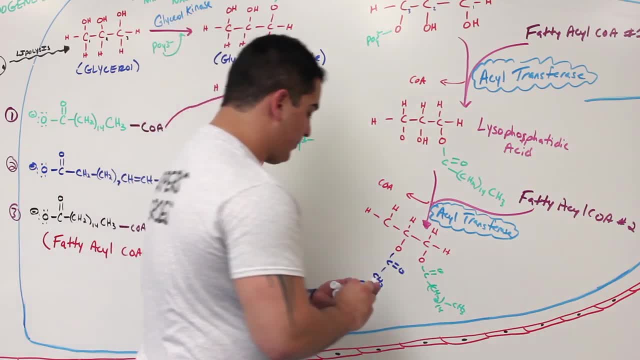 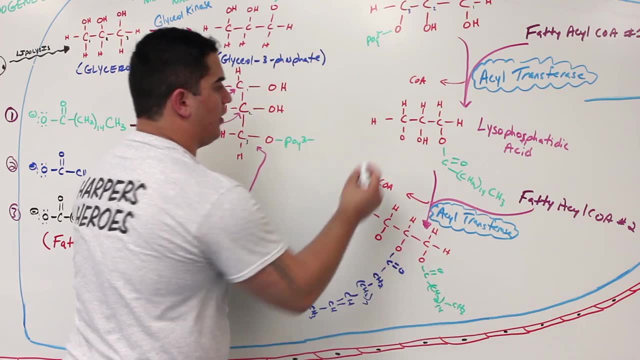 This is our next molecule. What is this guy here called? This guy is specifically: let's draw our oxygen here with the phosphate group. Need to be consistent with our molecule here. This should have a phosphate. This should still have a phosphate. 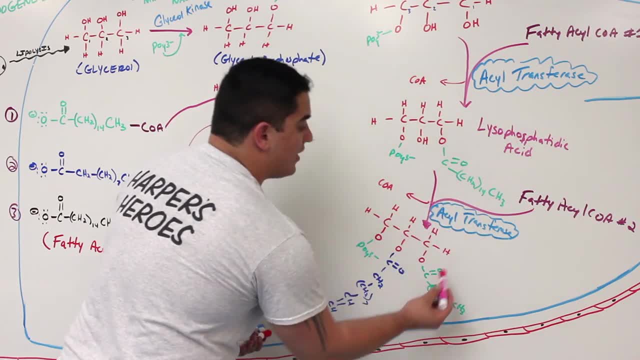 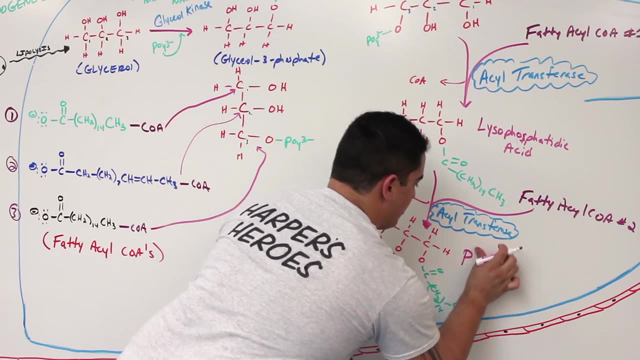 And again this one's called lyophosphatidic acid. This is just going to be called phosphatidic acid, So this molecule is called phospha Phosphatidic acid. I keep spelling my things wrong. 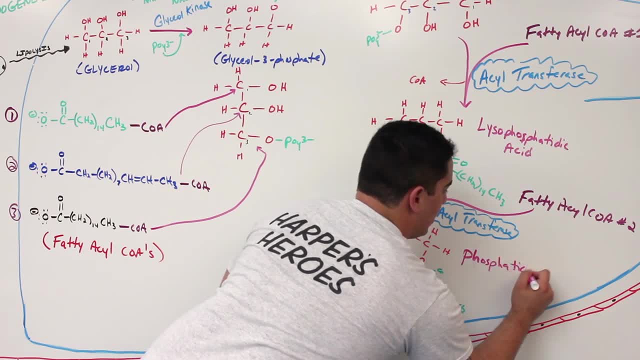 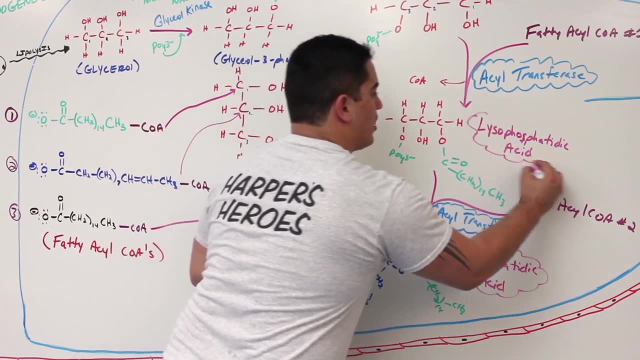 Phosphatidic acid. Okay, So we got phosphatidic acid, comes after, And then there was lyophosphatidic acid, And before that we just had the glycerol right As our basic unit. 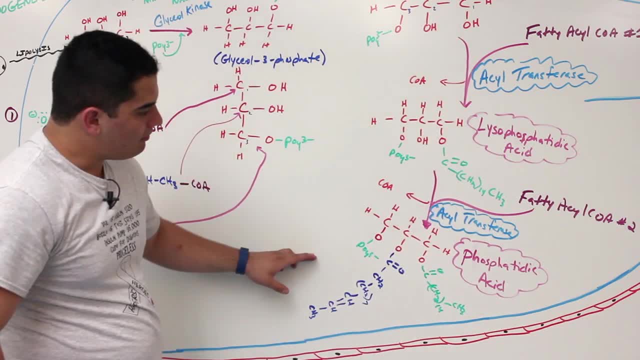 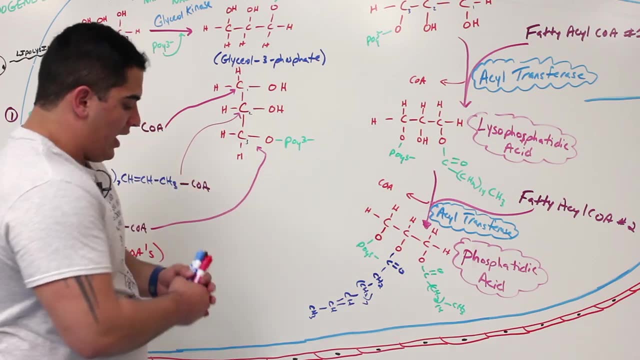 Glycerol 3-phosphate. Last step, Now what we're going to do. Actually, there's two more steps, but it's going to be simple. We're going to combine these two steps together. If I combine two steps together, 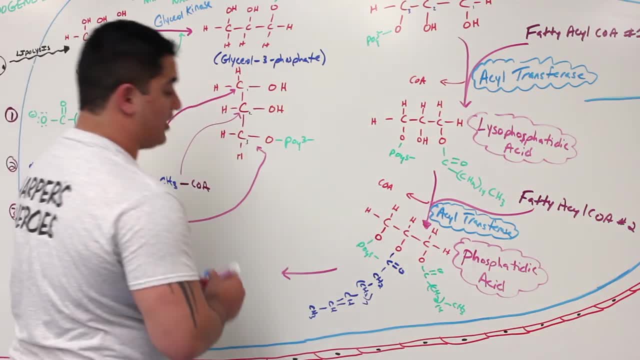 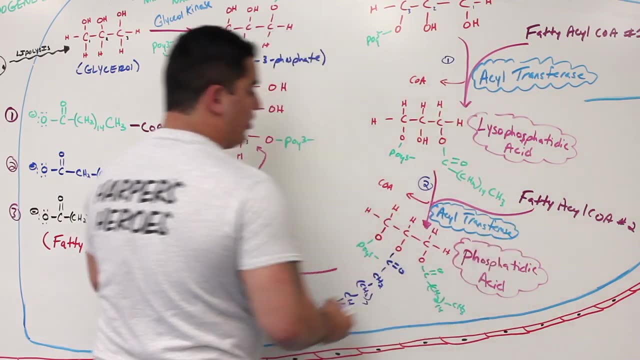 I'm going to do the same thing I did in the first two steps. So again, this was step one, where I added fatty acyl-CoA number one. This was step two, where I added fatty acyl-CoA number two. In the third step, I'm going to do two things. 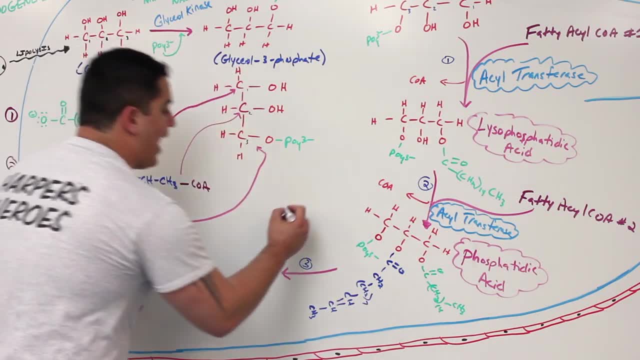 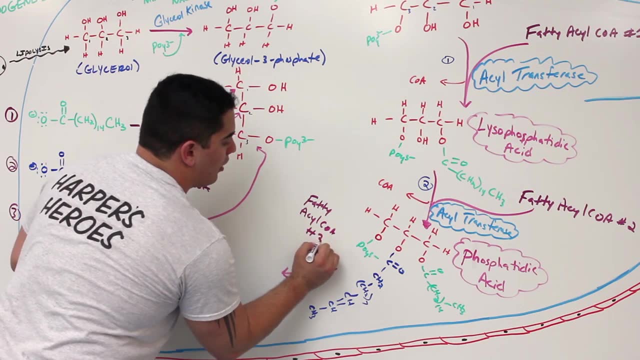 I'm going to add in what you guys already know. I'm going to add in my fatty acyl-CoA number three. I'm going to add this one in too. And what am I going to lose out of the process of this? 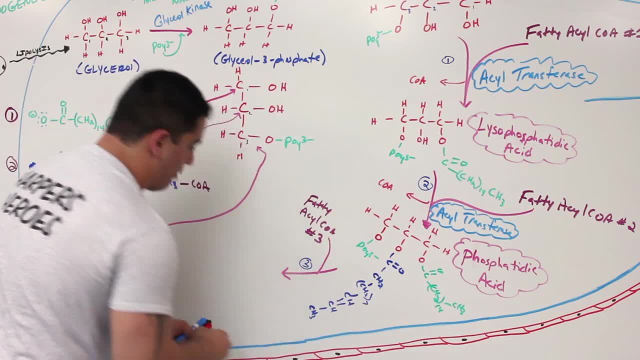 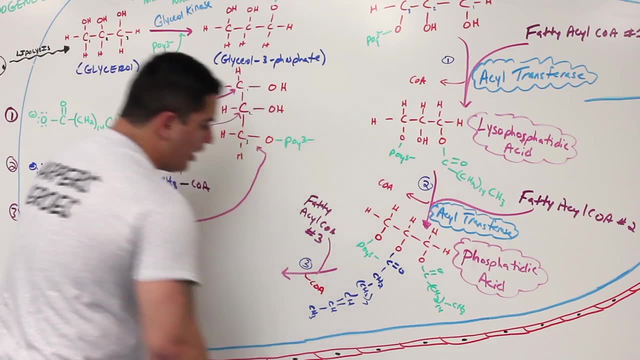 I will lose a coenzyme A. So I'll lose a coenzyme A out of this process. Coenzyme A, But here's the kicker. Look, can I add that fatty acyl-CoA onto this end? No, Because there's a phosphate there. 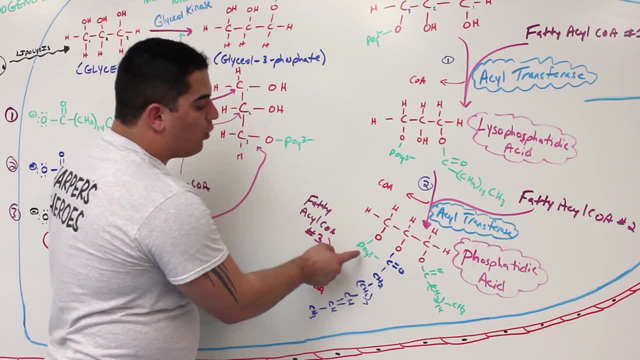 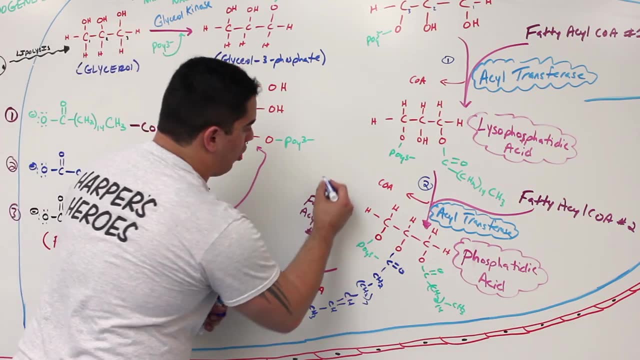 So I have to get that phosphate off first. So what do I have to do? before I add the fatty acyl-CoA, I have to bring in a special enzyme. What is the special enzyme? The special enzyme is called a phosphatase. 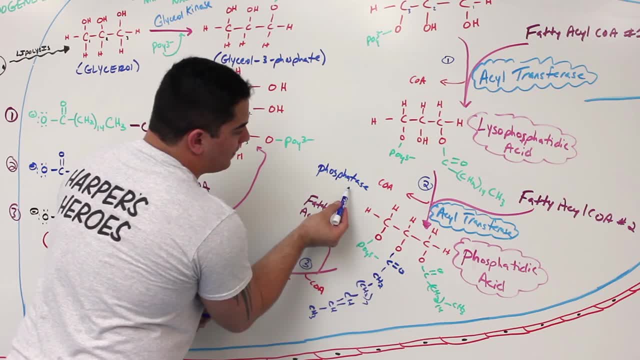 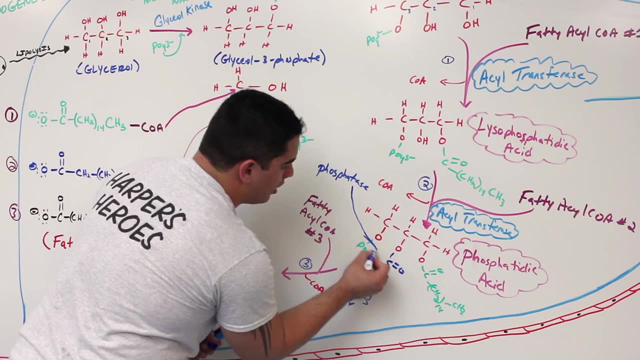 Phosphatase. And what's this phosphatase going to do? So technically it's a phosphatidic phosphatase. It's going to come in and it's going to cut that bond right there. It's going to cut this bond here and it's going to release out a phosphate. 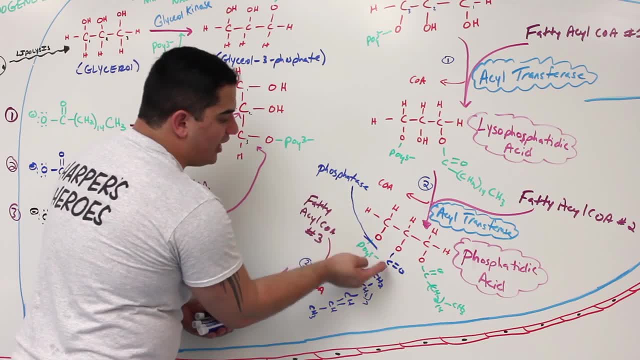 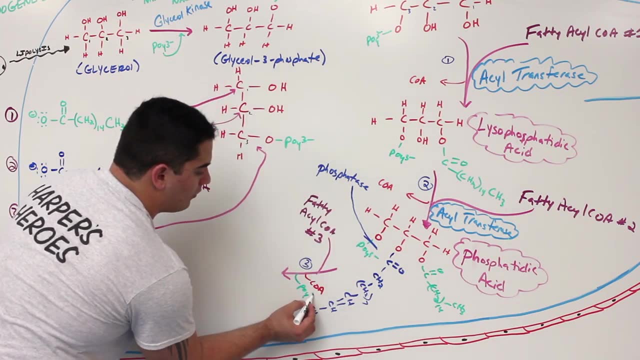 So again, what enzyme is going to do this? A phosphatidic phosphatase will cleave that phosphate off of the third carbon. So what am I going to release out of this reaction? I'm also going to release a phosphate. 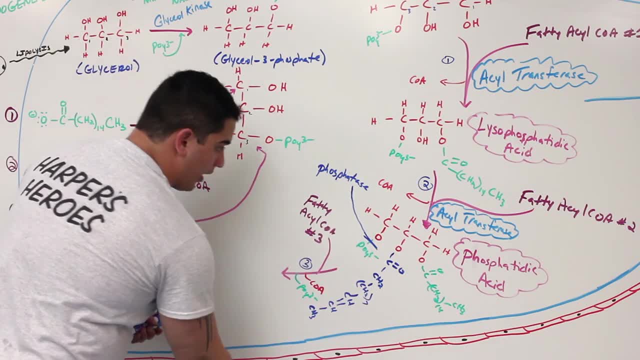 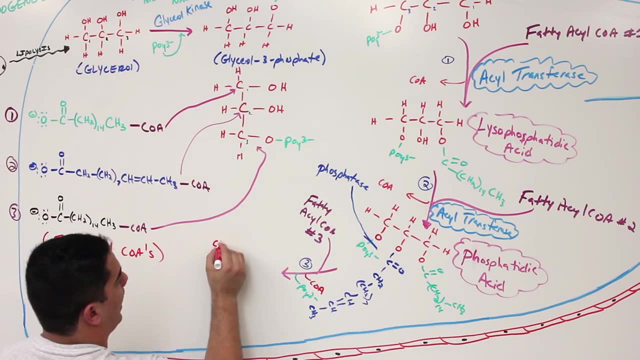 Then I'm going to add the fatty acyl-CoA number three onto the third carbon, here with the oxygen right. So now let's draw our finished triglyceride product. So again, I'll have- let's draw it here in an angle. 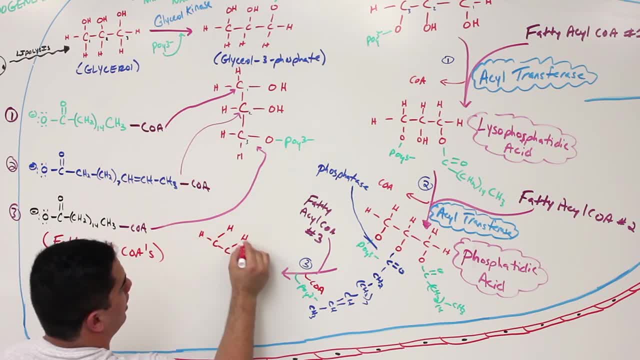 Carbon hydrogen, carbon hydrogen, carbon hydrogen and another hydrogen. And again, let me draw all my oxygens here And now. let's draw our finished product. The first one had specifically a carbonyl with a CH2.. 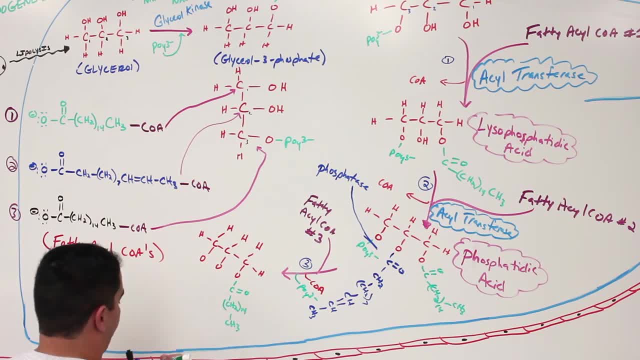 Fourteen of them like that, And then a CH3.. The second carbon had specifically what It had: a carbonyl with a CH2.. Then it had CH2.. Seven of them like that. Then it had a double bond And then a CH3.. 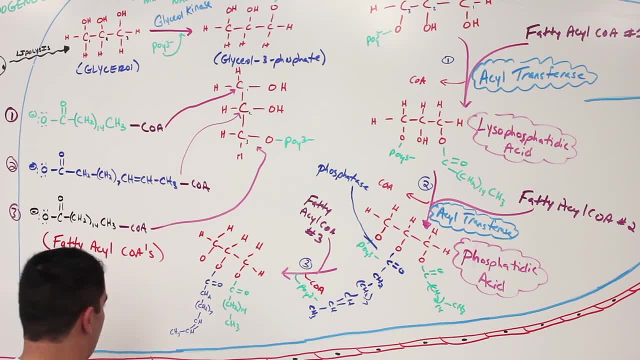 And the last one specifically had what. This one is going to be exactly the same as the first one. So what are we going to have here? Carbon double bond oxygen, CH2.. Fourteen of them like that, And then CH3.. 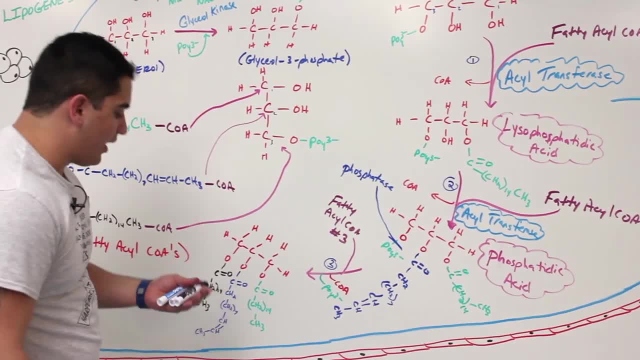 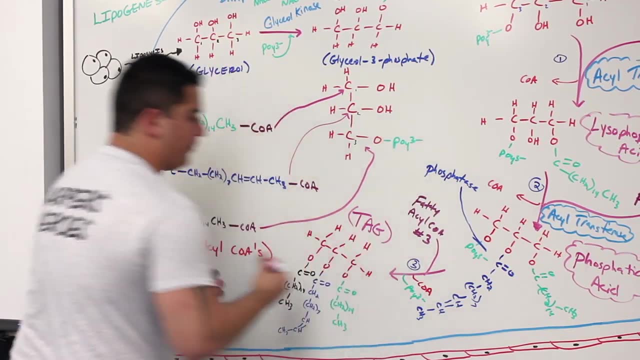 What is this molecule here called? This is called a triglyceride, But sometimes they refer to triglycerides. they give them a different name. They call it a triacylglycerol. Sometimes you might even see it referred to as a triacylglycerol. 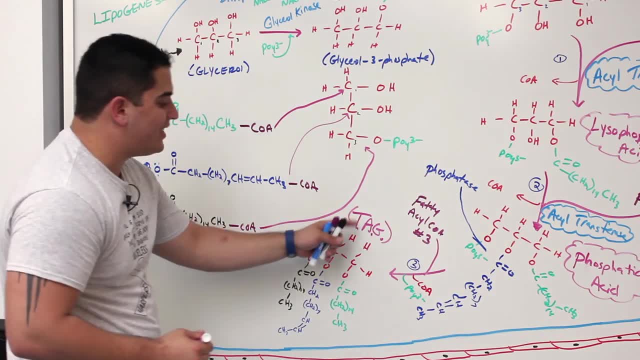 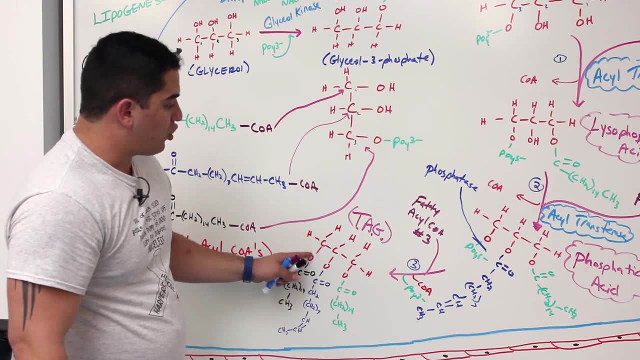 So be prepared to hear either one of those terms, Because a triacyl, this is a fattyacyl, this is a fattyacyl, this is a fattyacyl, So we're adding on fattyacyl groups, So you can call this a triacylglycerol. 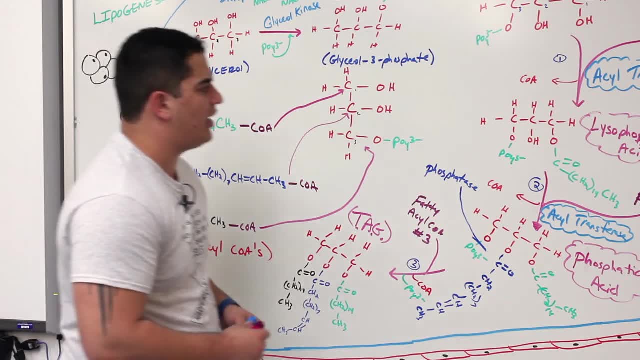 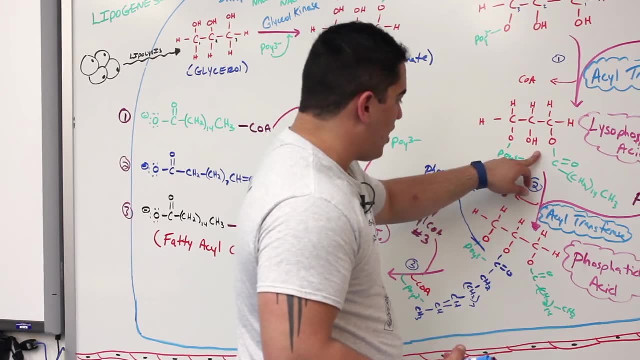 A acylglycerol or just a triglyceride, Because you know another way that we can name these Technically. this one is a specifically a monoglyceride or a monacylglycerol. This one is technically considered to be what 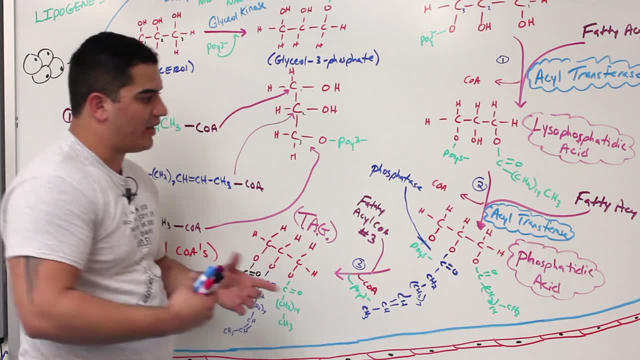 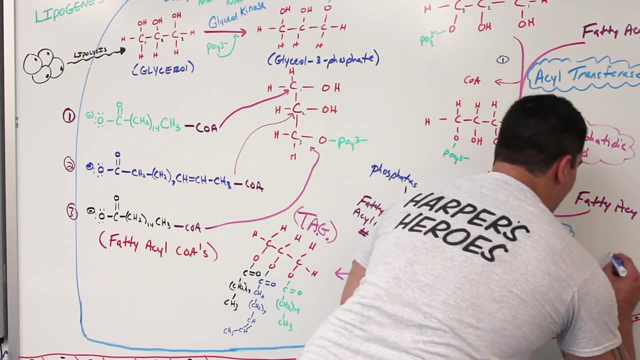 A diacylglycerol and this one is a triacylglycerol. So I can also kind of name these different names too, if I want to. I could technically call- I could call this one a DAG, which stands for diacylglycerol. 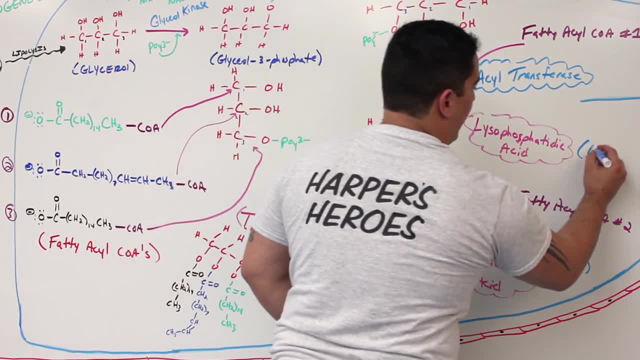 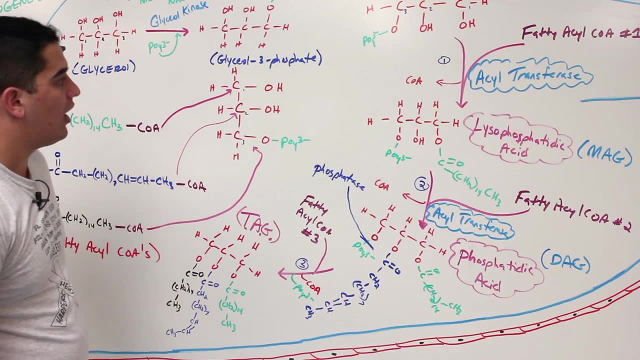 For this molecule right here, And I could technically call this one a MAG, a monacylglycerol, And again, this one is a triacylglycerol. Alright, so this covers the triglyceride synthesis. Now the next question is- and we're going to cover this- when we link this to cholesterol metabolism. 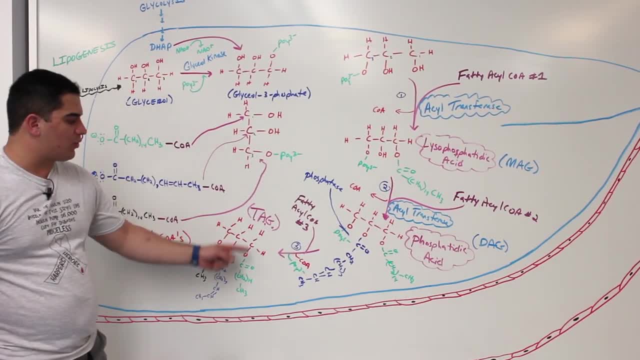 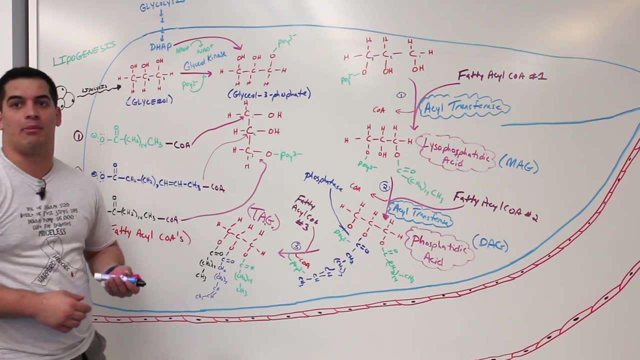 Is: what can I do with these triglycerides? Well, these triglycerides can actually be packaged into special, different types of lipoprotein molecules. Those lipoprotein molecules that we're going to package them in is going to be called very low density lipoproteins. 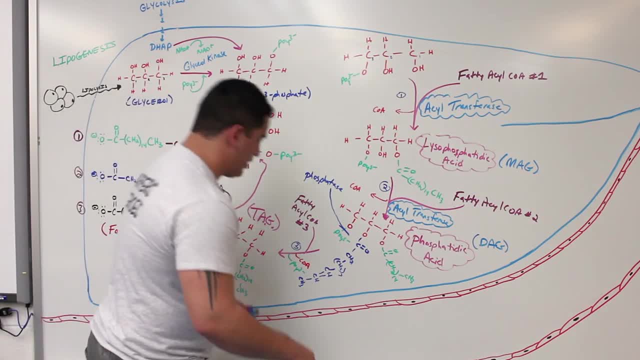 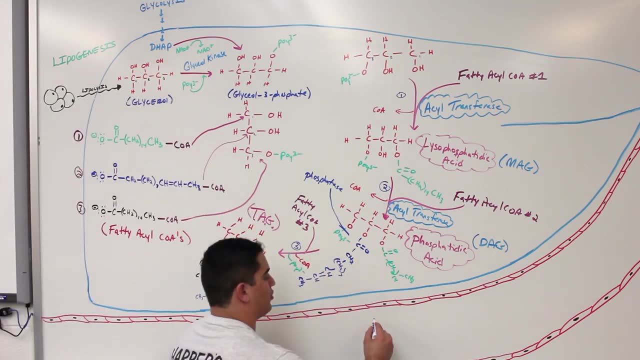 So what we're going to talk about in another video is specifically me taking this triglyceride and packaging them into special structures. And again, what is these special structures? Let's say, I draw it here And I can put this whole triglyceride, which I'm going to just draw now, in a different way. 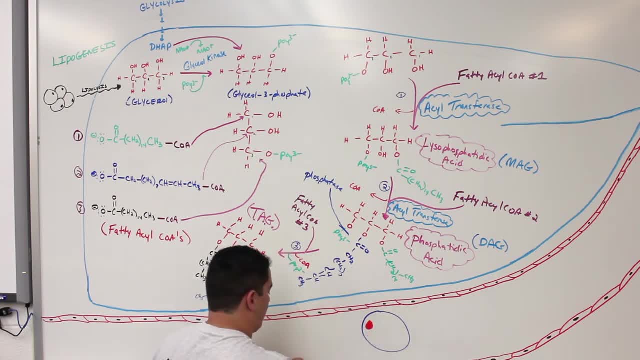 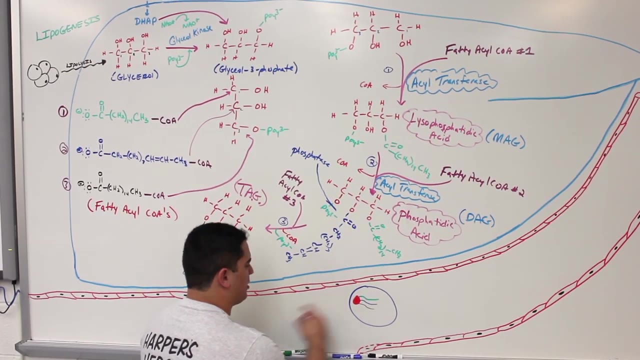 But meaning the same concept here. So now let's have a green fatty acid, We'll have a blue fatty acid And we'll have a black fatty acid, And this is going to be in a specific type of lipoprotein molecule With specific types of apoproteins, which we'll talk about. 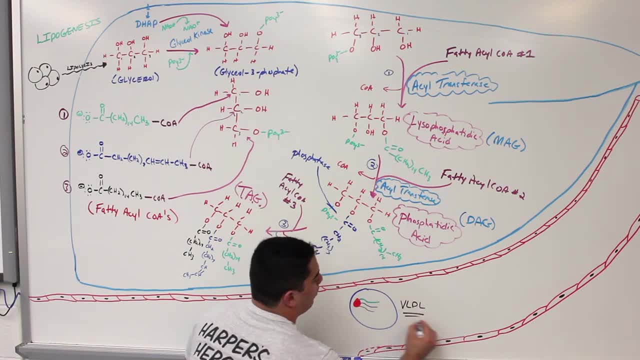 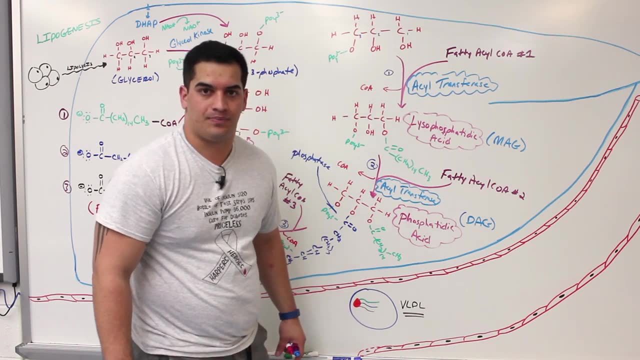 And this is going to be called a VLDL. And where can this VLDL go? It can take and transport this triglycerides and a tiny little bit of cholesterol to adipose tissue, Where it can be deposited into the adipose tissue and stored as triglycerides. 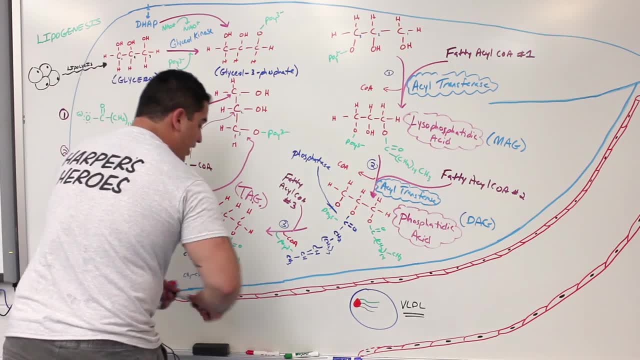 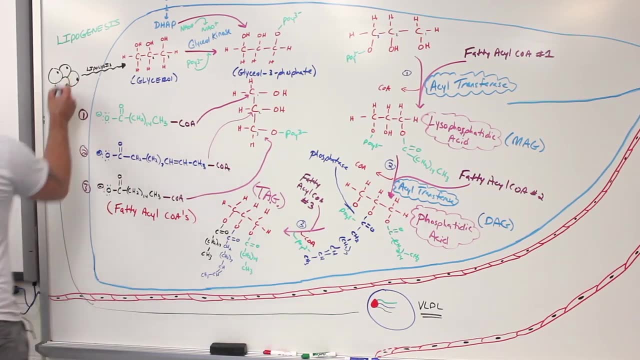 So again, where could this VLDL go? This VLDL could come over here, Where It could come over here And do what It could: be: transported through the bloodstream And then deposit those triglycerides into the adipose tissue. 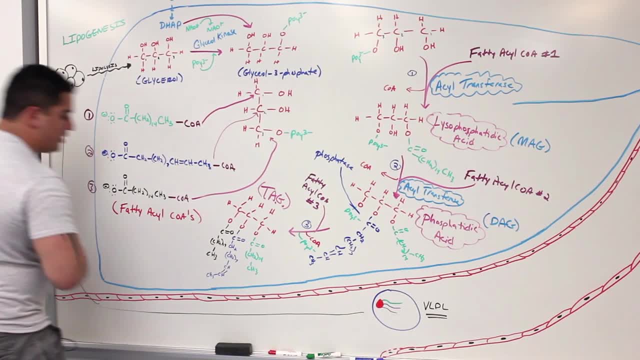 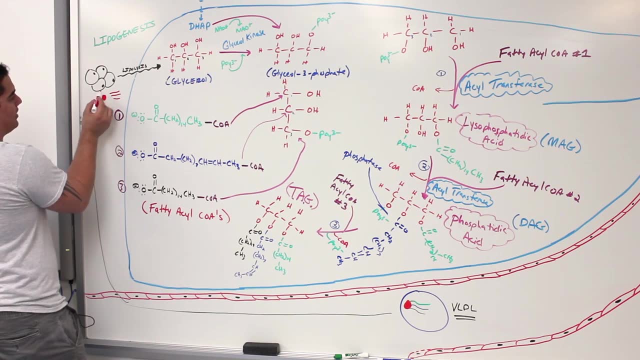 So what is it going to throw in here? It's going to throw into the adipose tissue. I'm just going to draw it here in a general way. guys, It's actually going to get broken down by lipoprotein lipase, But what's going to happen is it's going to get taken into these adipocytes. 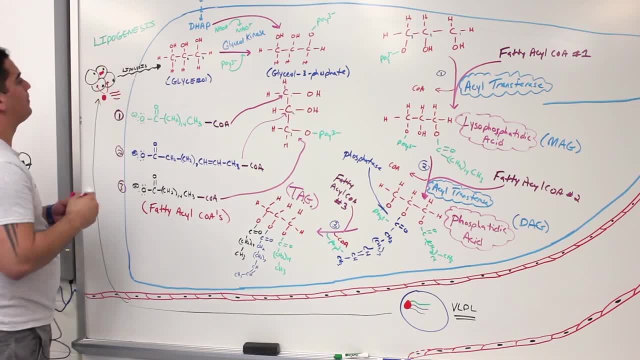 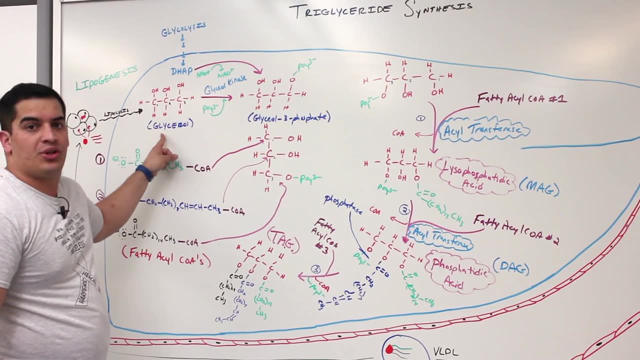 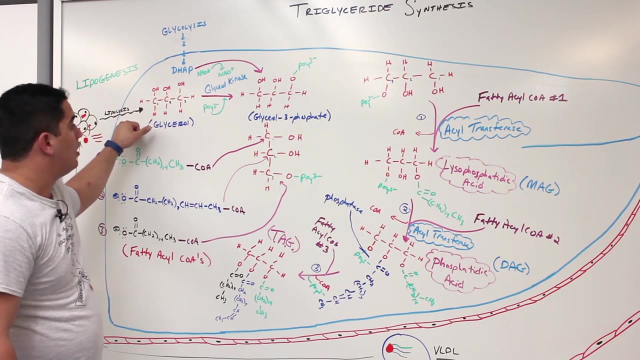 And then resynthesized back into triglycerides Where they can be stored. Okay, So just a really quick recap. Again, we need glycerol as our basic unit, Which can come from glycolysis, from the DHAP, Or it can come from the actual breakdown process from the adipose tissue, like lipolysis. 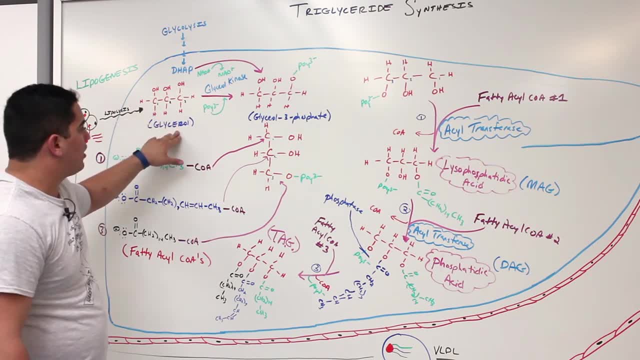 And again, this also can happen a little bit in the liver, but not too much. But then the glycerol. what can happen? Only in the liver? you have this glycerol kinase enzyme Which does what? Converts the glycerol into glycerol 3-phosphate. 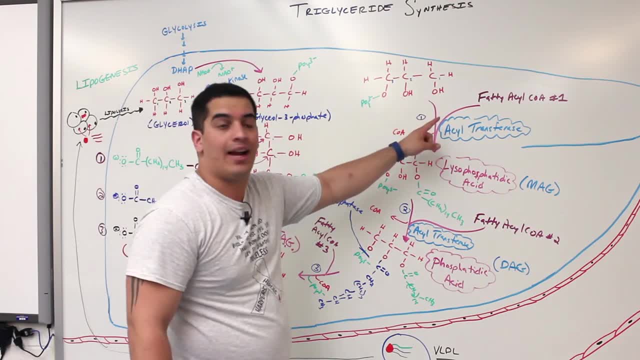 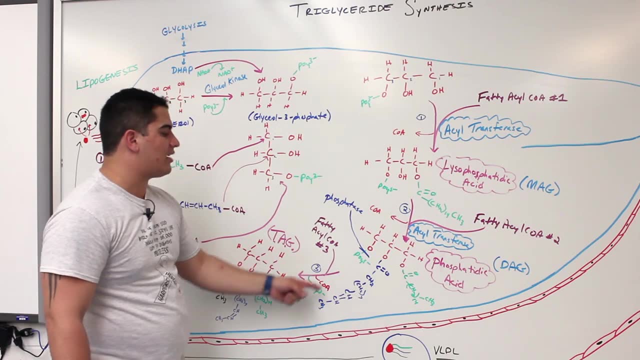 Which is the basic unit for what? For these fatty acetyl CoAs to be added. And what did I do? I added each fatty acetyl CoA in a sequence: One, Two And three, And again what would be the enzyme I didn't mention here? 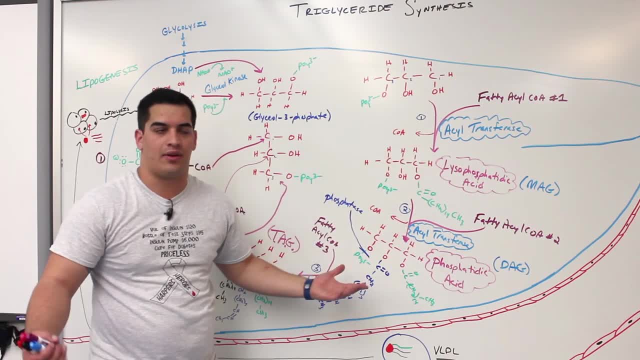 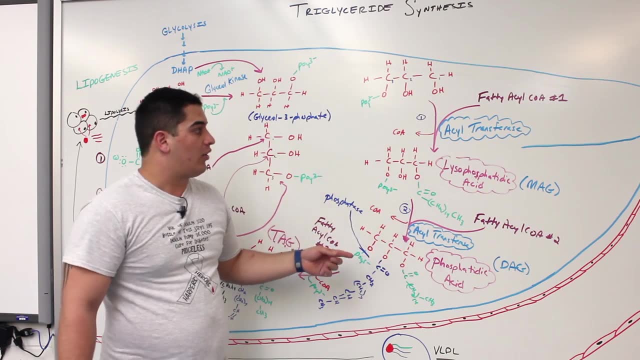 But it's the same enzyme that we mentioned in all of these Acetyl transferase in the third step again. But all you're doing is you're adding these fatty acetyl CoAs in sequence with an acetyl transferase present. Okay, 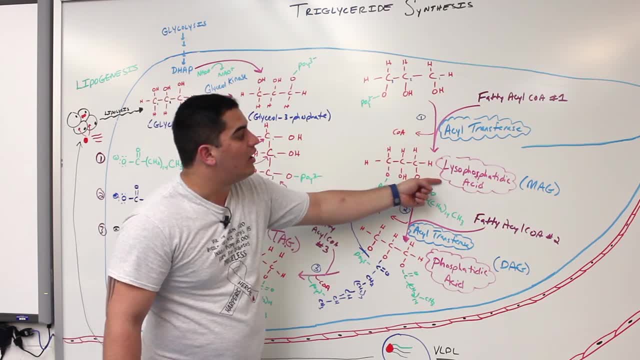 Converting it into what? So taking glycerol, Adding a fatty acetyl CoA And going into lysophosphatidic acid or a mono acetyl glycerol, Taking that lysophosphatidic acid or the mono acetyl glycerol. 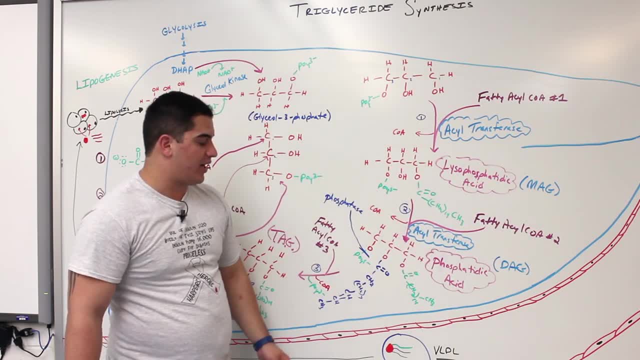 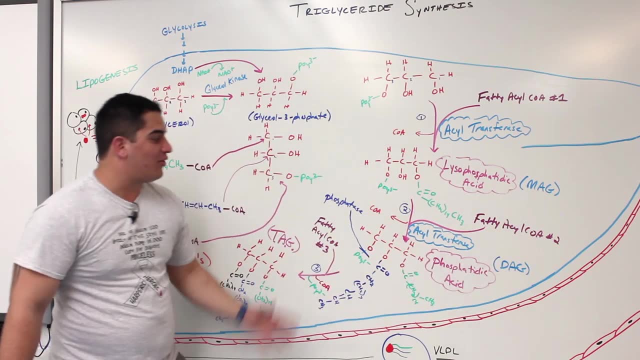 And taking another fatty acetyl, CoA, Adding that in with the acetyl transferase And forming phosphatidic acid or a diacyl glycerol. Taking that phosphatidic acid and diacyl glycerol, Doing what? 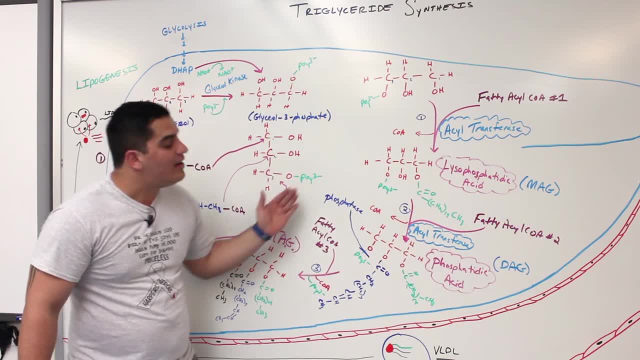 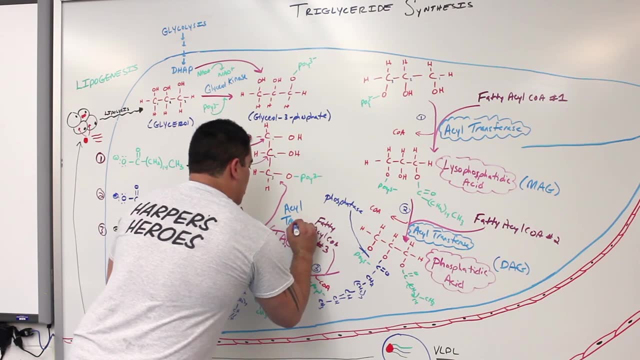 Getting rid of the phosphate with the phosphatase enzyme And adding another fatty acetyl CoA with another. what? What is that enzyme? again, in this step, Acetyl transferase. And again, what do you form? You form a triacyl glycerol.